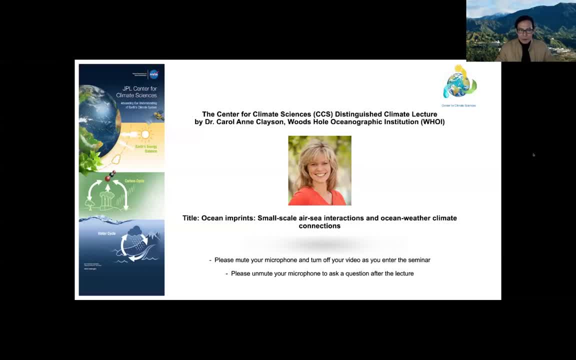 2018 and 2019, and on the butterfly proposal since 2013.. and without further ado, please welcome carolyn to present the ccs distinguished climate lecture. thank you, karen. thank you, tony. i'm going to work on this, sharing my screen now. um, when i was first asked to do this, i think it was pre-covered. 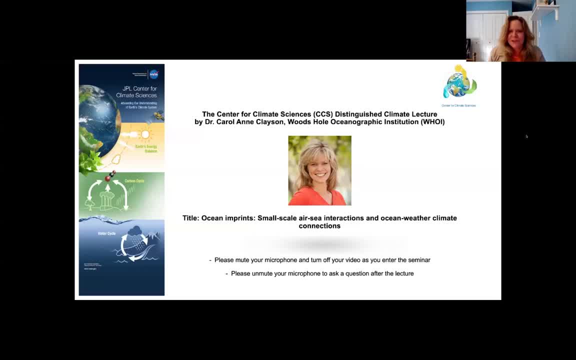 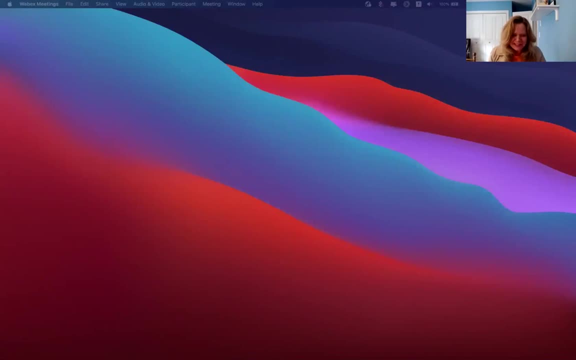 and i kept putting it off because i really much prefer being in person to give one of these. and then also i i knew it was a chance to come to jpl and and meet with you, um, but it's kind of dragged on and so, uh, that seems to be what we need. we just needed to do this. 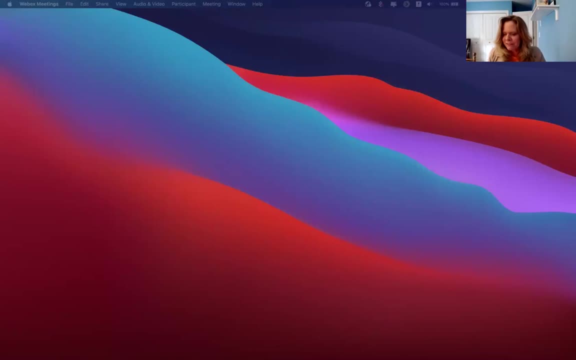 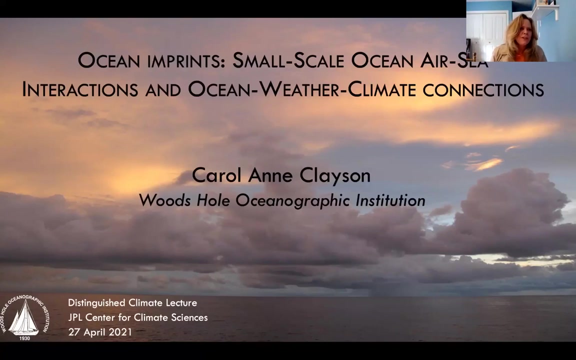 so i'm going to go ahead. i think you're seeing kind of a blank screen. well, it just background screen at the moment and i'm going to switch this off screen. all right, hopefully you're seeing a full screen now of my title page, is that correct? 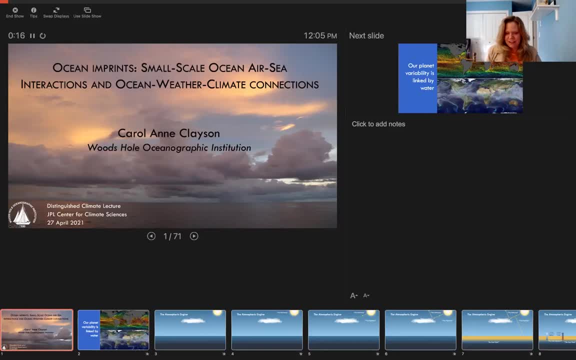 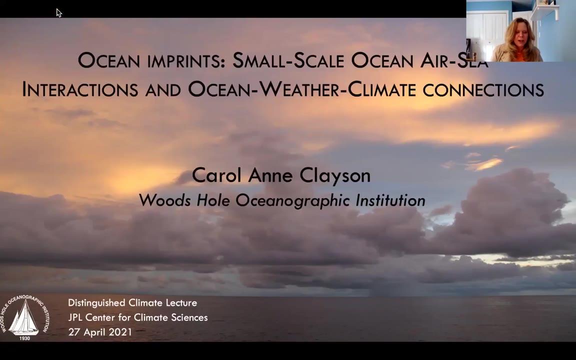 no, actually you had it right. uh, it was, you just switched it. yeah, oh, okay, it was right. okay, so that's good to know that it remembers what i did the last time. okay, now, okay, now it's a full. now is it a full screen? yeah, yes, it is okay. great, so, um, uh, again it's. 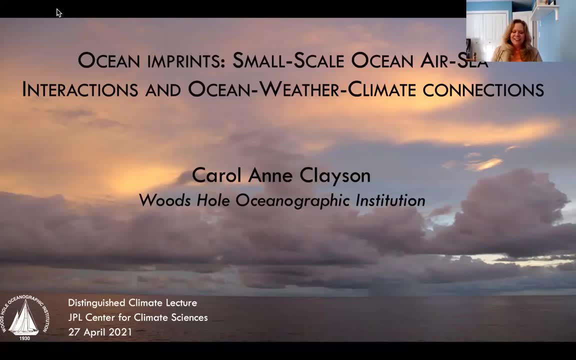 really my pleasure to be talking with you today. i i've gotten a few different um comments from various people about what i should try to do, up to and including sort of everything about how the ocean impacts climate. um, in sort of a general sense and then very detailed on my 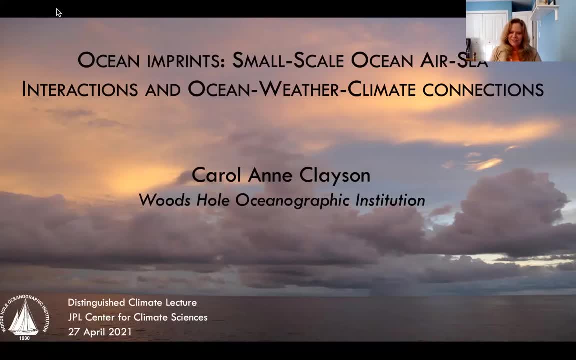 research, uh, and so i i kind of put those two things in the chat box and then i'm going to put things together which sometimes it may be more successful or less successful. i anticipate that many of you will already know um much of what i'm saying, just just because i am trying to give some 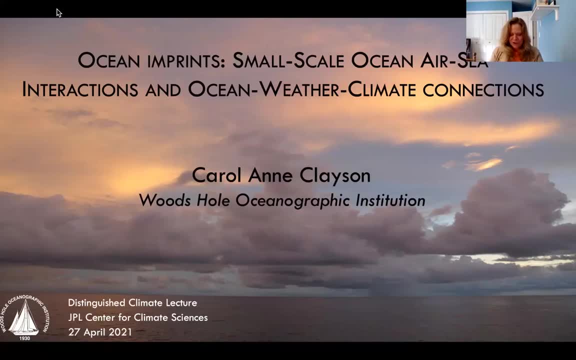 general context as well, but hopefully there's something useful for everyone. this is a picture that i took out on the spurs 2 cruise and i'll actually show a few results from that cruise. um, but i like. i like this figure because, first of all, it was great weather, really enjoyable it was in the tropical eastern pacific. 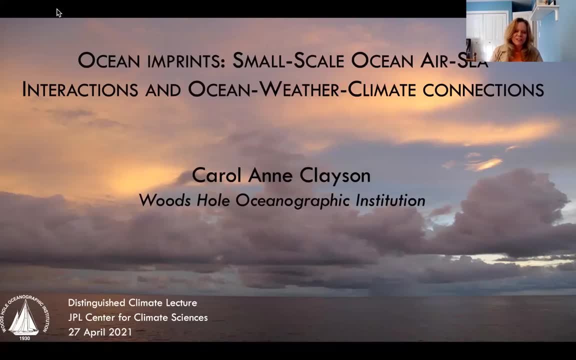 um, in summertime. so it was. it was very nice, but you can see just the highly inhomogeneous nature of the clouds. there's a little rain event going on over here, um, and it it sort of highlights some of the things that we're going to talk about and, again, if you have a question, i it'll be hard. 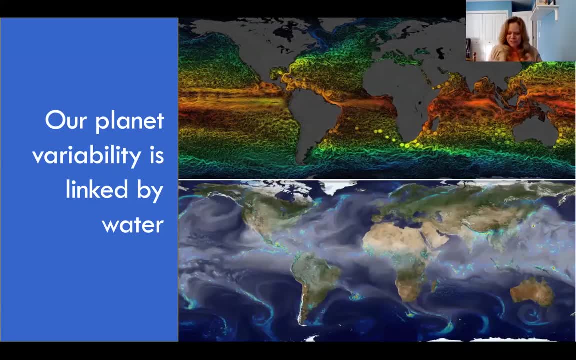 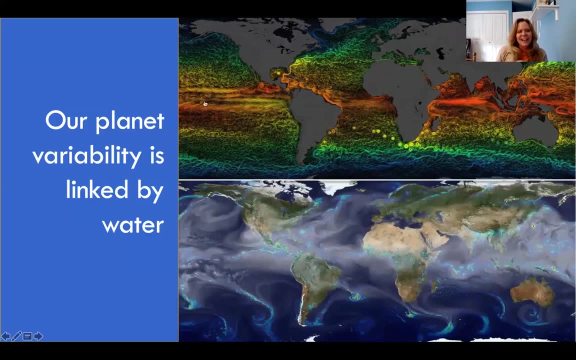 for me to see if you just raise your hand, so if you just unmute and just shout it out, that's you know, that's okay. that'll be easier if you, if you have a big question. so one of the things that i i actually end up doing quite a bit is i talk to a number of different groups. 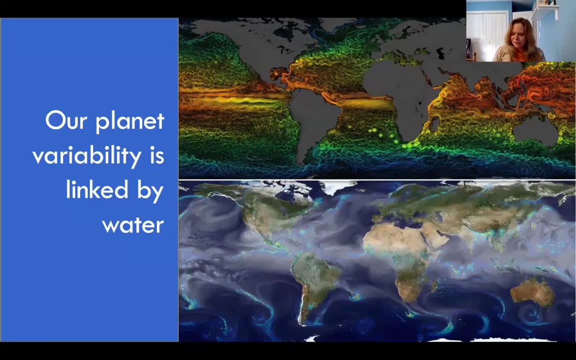 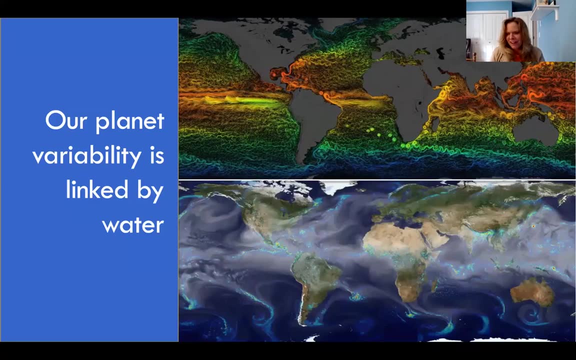 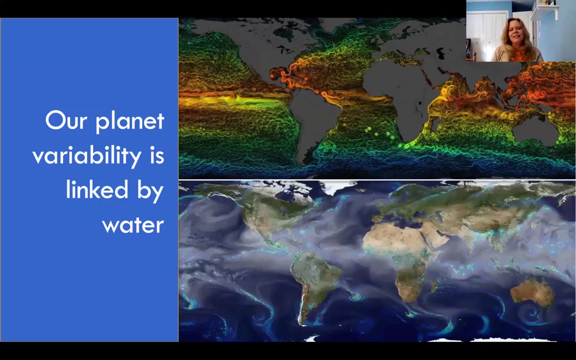 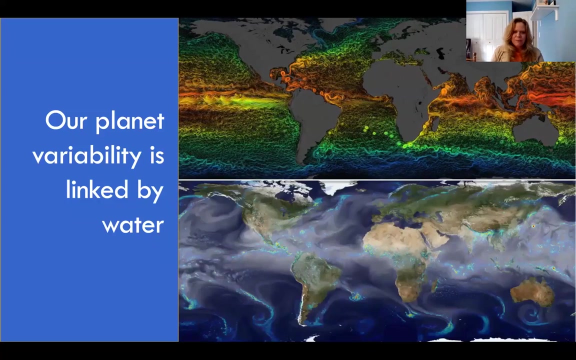 i i actually speak, even on occasion, with executive boards at large companies. i'm talking to one in july in and it's on climate, climate variability and this is one of the things that i like to do. that kind of demonstrates why we talk about the ocean so much, because often when i'm talking with various groups and they, they don't think. 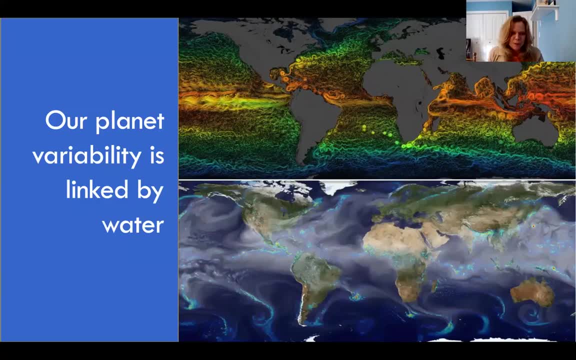 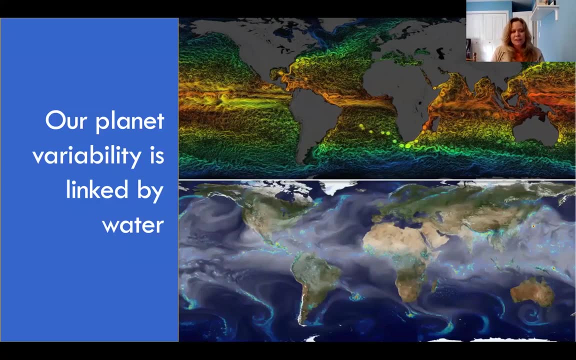 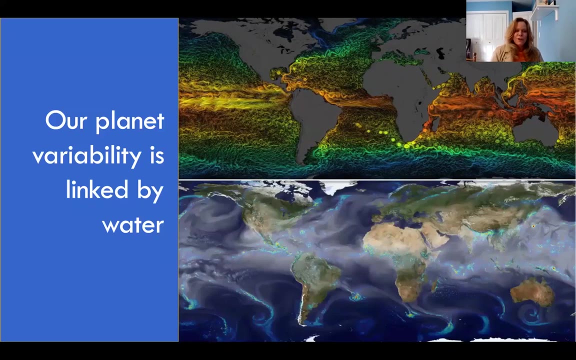 of the ocean really and how it interacts with climate and why it might be an important thing. but so this is now. these are two. these are two model simulations. the upper panel is surface current and the color then is the surface temperature, and so you can see some of the great features of our, you know, our whole ocean circulation system. you can see. 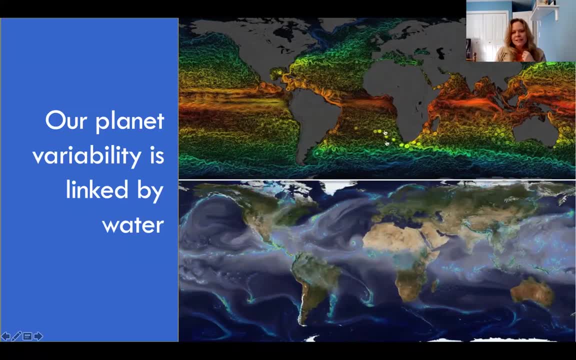 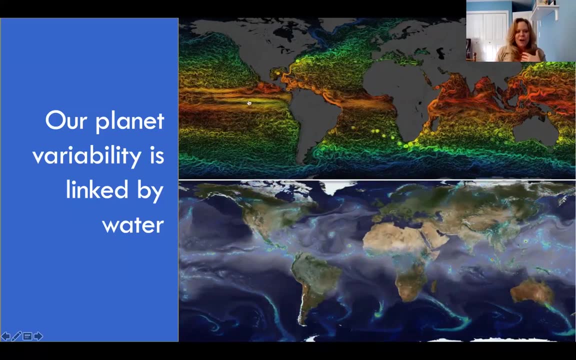 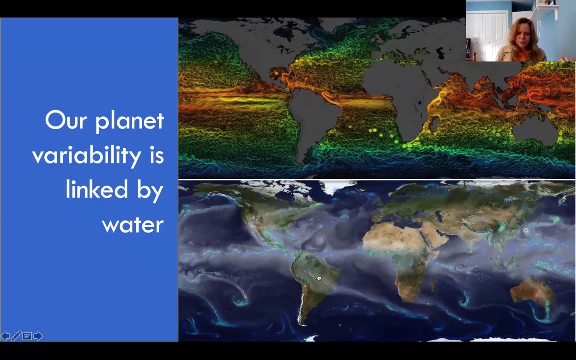 the gulf stream. you can see the agulhas currents and eddies circles here. you can see some of the waviness here, the tropical instability wave. anyway, you can see a lot of different features. on the bottom is atmospheric water vapor and i like to say our planet variability is really linked by 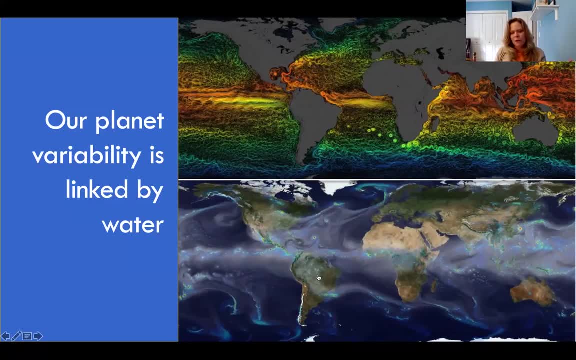 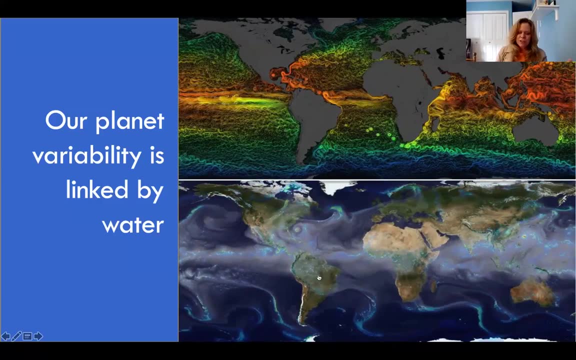 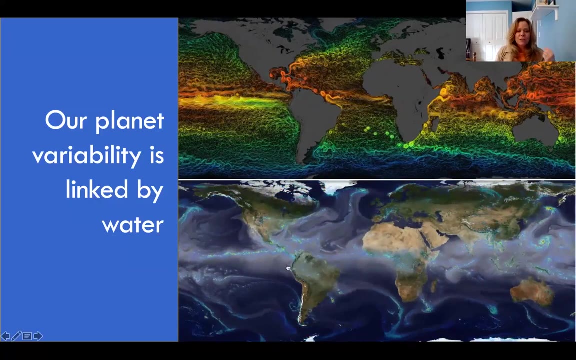 water and, in fact, when i talk with outside groups about, about climate, we do talk about the fact that you know that water is really the expression of the climate change that is is going to be most perhaps impactful um for for people to see. so i like to, i like to demonstrate. 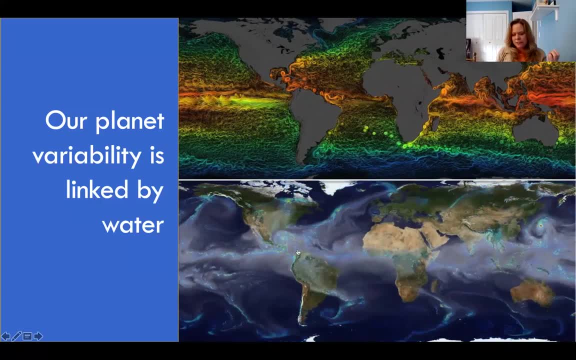 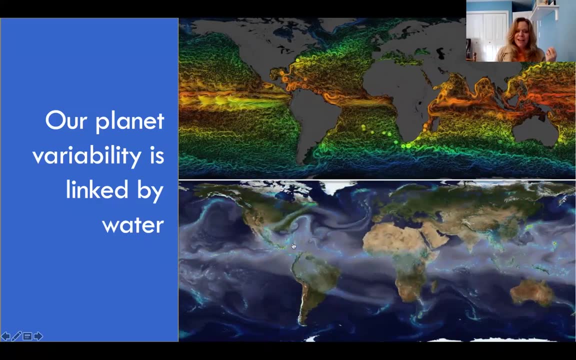 this just because you can begin to see how, how closely linked the two, the two fluids, the atmosphere and the ocean, are linked by by their water and the variability and where the water is in the atmosphere and you know how it, how it changes, um has a lot to do with, of course, the 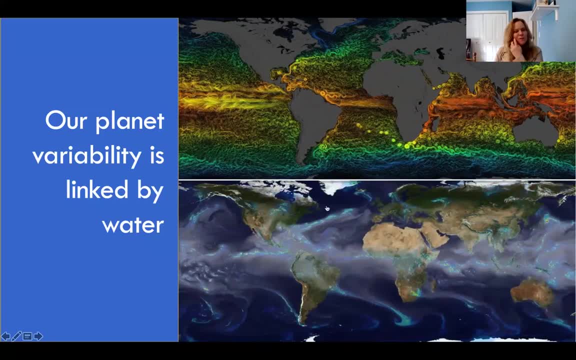 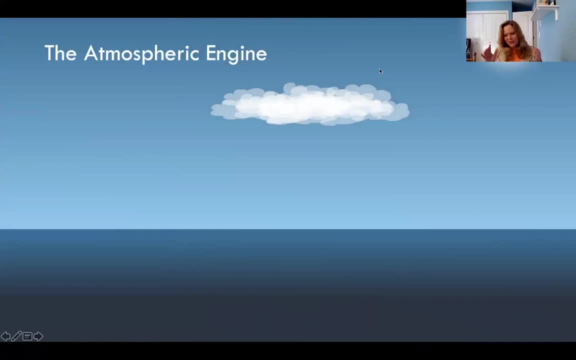 ocean current, um, although the atmosphere is moving much more quickly than the ocean. so one way that i like to think of what i do, which is really look at how the ocean and the atmosphere interacts, is i. i like to think of it in terms of an engine, um, and i like to 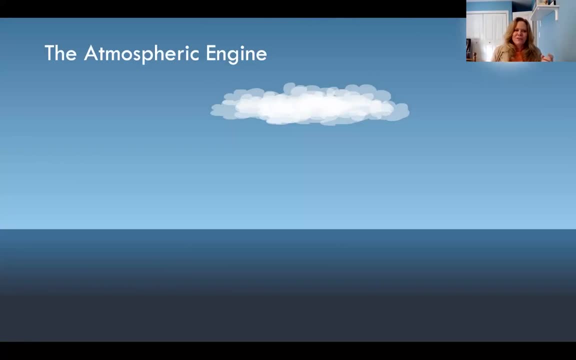 think of the whole atmospheric engine. so first we have the refinery, which is the sun, and then we have the sun's energy coming through the atmosphere. there's a pipeline that energy is transferred to us and it's a little bit of a leaky pipeline if you're thinking about how much energy actually gets down to the surface, but indeed a large amount. 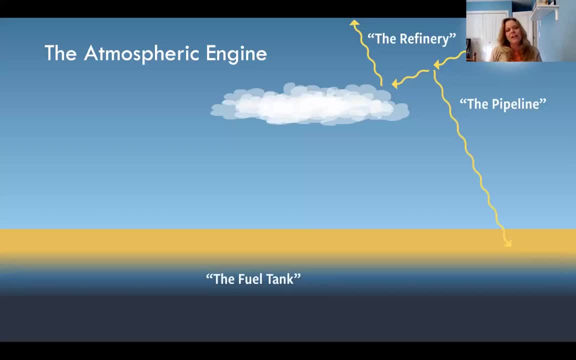 of the energy makes its way through the pipeline into the ocean and heats it up, and so the ocean then essentially becomes the fuel tank for the atmospheric engine. and then i like to relate the turbulent exchanges of moisture and heat between the ocean and atmospheres to the fuel injectors of our, of our atmospheric engine, so that the 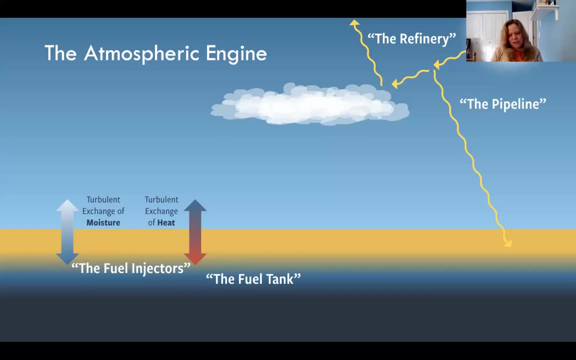 uh, the fact of the ocean, on average, is warmer than the than the atmosphere, and also, on average, is more moist than the near surface atmosphere, means that there's a lot of exchange of heat and moisture from the ocean to the atmosphere and that creates more moist air and it warms the air. 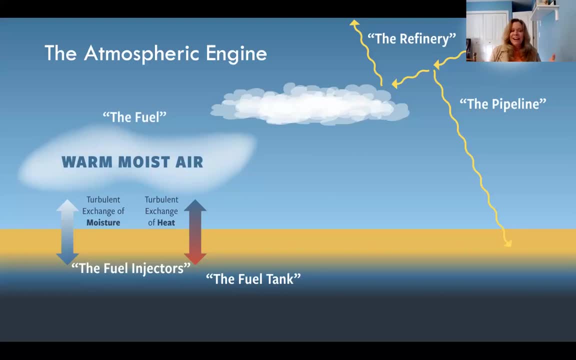 and moistens the air. and that warm moist air then is basically the fuel of, of our atmosphere engine. and once we have that fuel injected into the system, the wind which is moving that warm moist air throughout the, throughout the system, and in return the wind drives through the turbulent exchange of momentum, drives, waves and currents in the upper 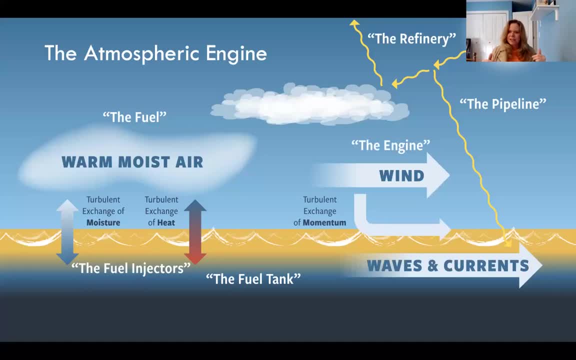 part of the ocean, and one of the things that i like to think about when we talk about that is that that turbulent exchange of momentum between the wind and the ocean is really the break of the atmospheric engine. so we've got the fuel injectors and the brakes and some of what we are trying to. 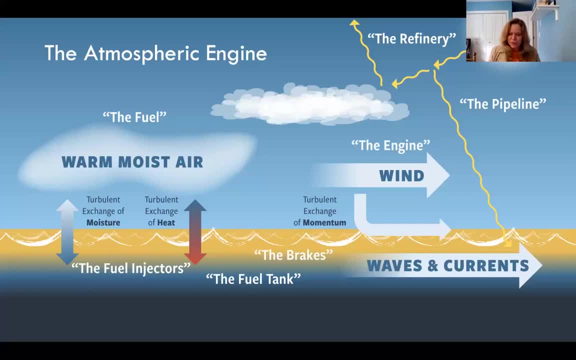 understand is sort of what is the ratio of the fuel injectors to the brakes? this comes up particularly- people have come across this discussion- in things like hurricanes and hurricane intensification. so there's, you know, the injection of energy through the heat and the moisture exchange, but there's 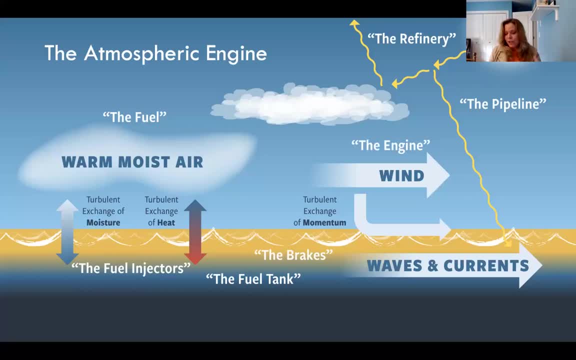 also the brakes on the hurricane through the, through the loss of momentum to the ocean surface and- and although i'm not going to talk about it today- really understanding how to model that exact phenomena, especially at high winds, is something that we're kind of lacking on, but today i'm going to. so this is just sort of an overview, to place you in the context. 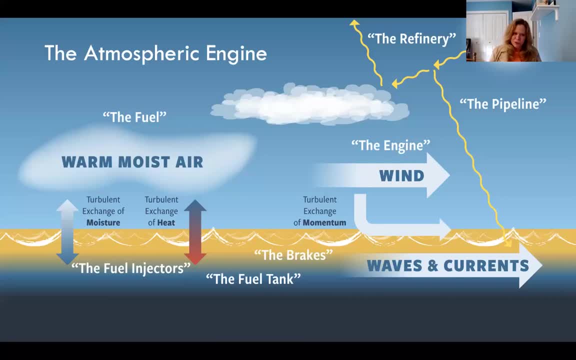 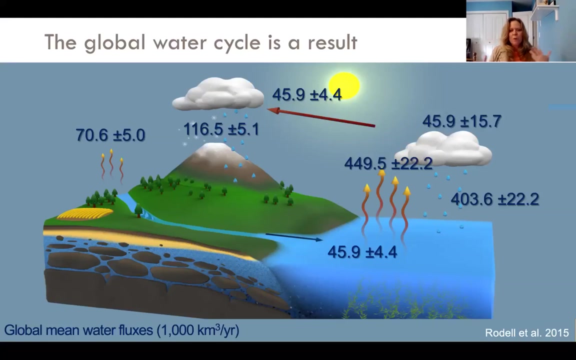 of why i'm going to spend a great deal of my time talking about the turbulent exchange of these products of moisture and heat and looking at the fuel injection, but as we see how this energy and moisture is exchanged between the ocean and atmosphere, one of the things that's a 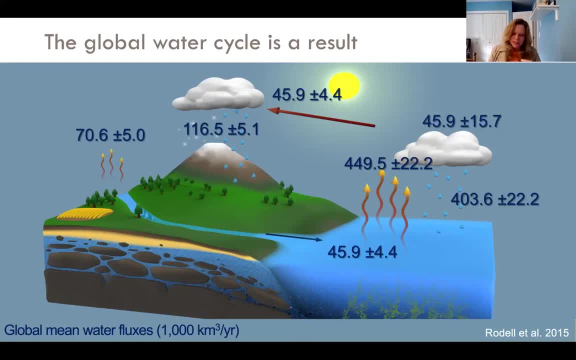 result is the global, global water cycle, and this is a a great paper by matt rodell. there's a companion paper by tristan lecrier, which is: um. essentially what they did is they took almost entirely uh satellite data- that was modeling, reanalysis for atmospheric divergence, but 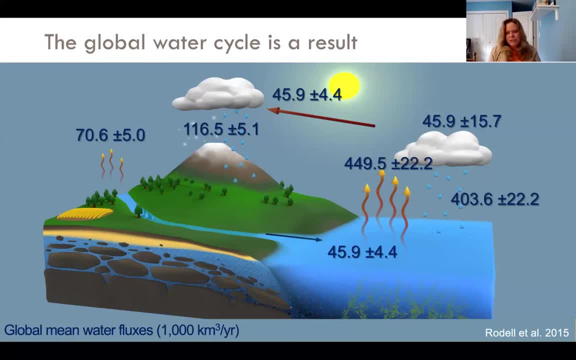 they took all of this data, put it together and then put it in this data, and then they put it in the And did a very nice quantitative balancing to try to try to determine what is the optimal, Uh correct that we think should be happening in the various components of both the water cycle and the energy cycle, because the linkage between those 2 is the latent. 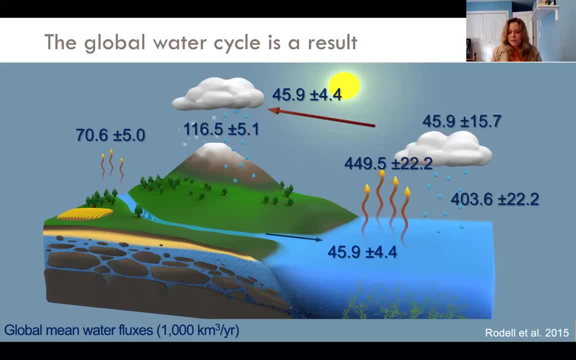 Heat flux, so it's an exchange of moisture between the ocean and atmosphere, but it's also an exchange of heat. So 1 of the 1 of the things that they did- that was that was really quite well done- was Putting those 2 together and balancing them at the same time. 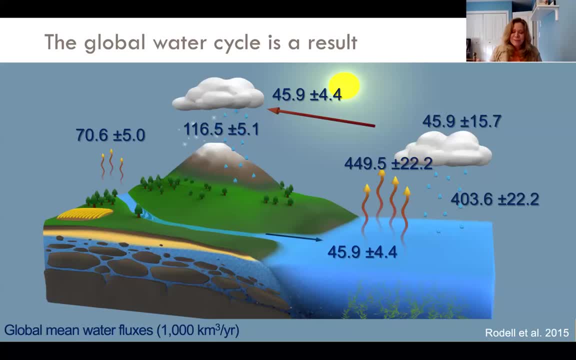 Making sure that the latent heat flux was consistent between the 2, and they were also very careful and taking uncertainties from the various products And this is sort of the balance that that has gotten this. and again, because I was speaking to a bunch of oceanographers, we would, we would spend a little while talking about why they they use. 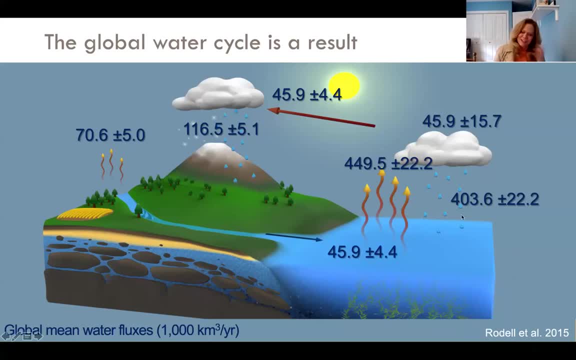 1000 cubic kilometers per year, but I just kind of land people and let the numbers go. Okay, All right. So in these units, the largest number that you can see here is is The global ocean of operation at almost 450,000 cubic kilometers per year. 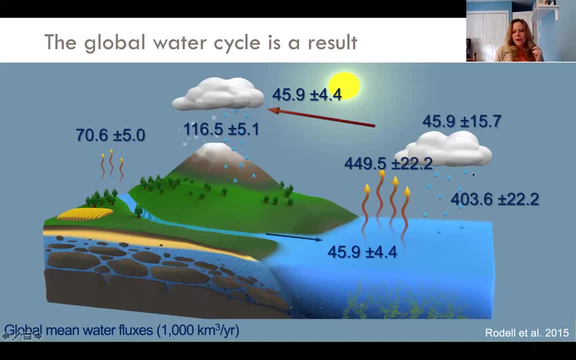 And you can see it's larger than The ocean over ocean precipitation. that of course, then leads to an infection of moisture to over the land. There's the, There's the river. run off here some latent heating evapotranspiration as well from. 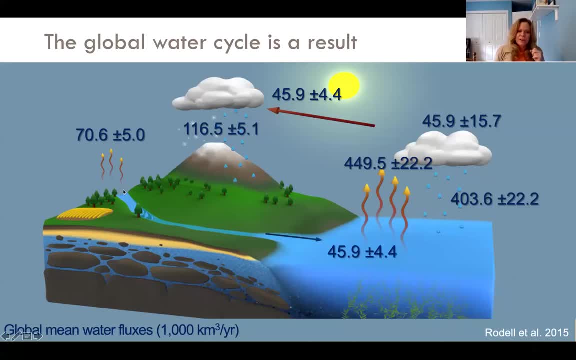 From the plants and the land surface and lakes and so forth. So 1 of the reasons that I show this slide- and I will show this again because there's a 2nd point that I'll make later on in my talk- 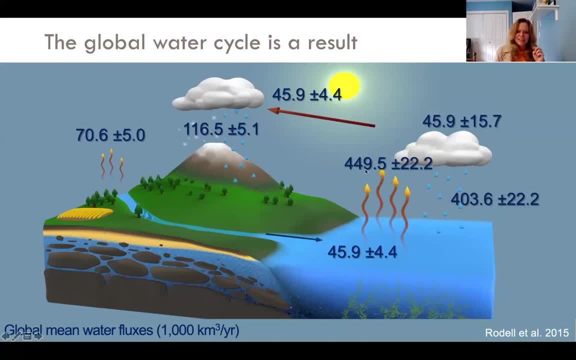 But In this particular 1, I do like to say this: This number right here is the single largest number in the entire global water cycle and it has 1 of the largest uncertainties as well, And we're going to talk about that a little bit more. 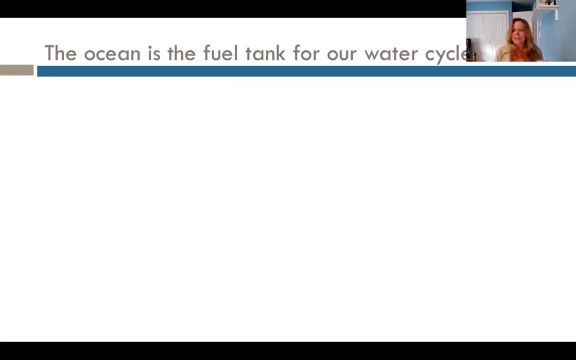 So again, so the ocean is the fuel tank, basically for our water cycle. We know that ocean evaporation supplies about 90% of the water vapor that eventually becomes rain, snow- About 40% of the rain and snow falling over land. 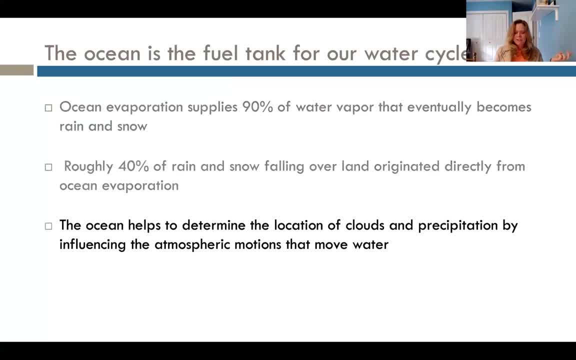 originated directly from ocean evaporation. The ocean also helps to determine the location of clouds of precipitation by influencing the atmospheric motions That move waters. we've talked about and a number that I I use, because sometimes I, when I'm talking with various other groups, we talk about the importance of the water cycle, sort of wherever you live on the planet, And 1 number that I do like to mention is that 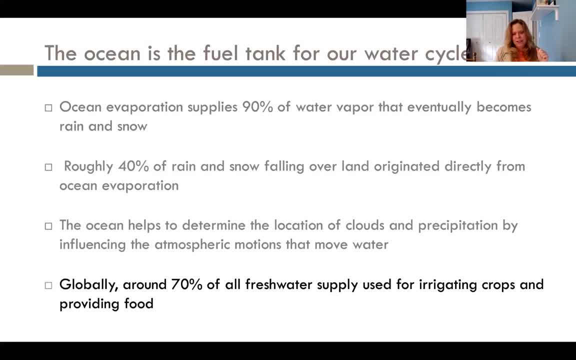 Globally, about 70% of our entire fresh water supply is used For air, creating hot crops and providing food, so changes anything that changes then in our water cycle that affects our fresh water supply, Um has an outside impact on on crops and food production. 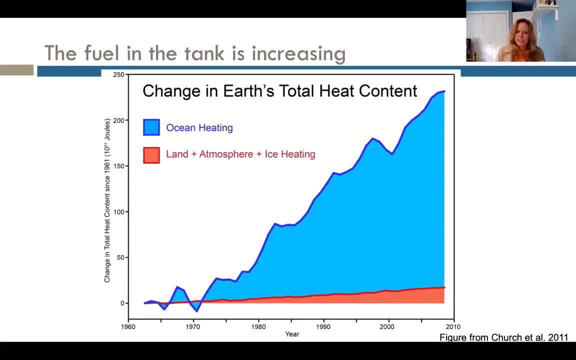 So the other thing that we know, of course, is that the fuel in the tank is increasing Um. this is a figure from church at all in 2011, and what we see here, this is often. I use this because I talk about what we see in terms of the change in your 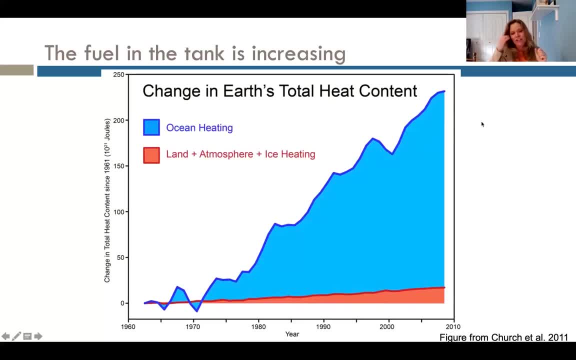 Surface air temperature globally and how that's changing and how this. this number is a much more unambiguous Indication. so this is of the of the extra heating that is being kept within our earth system. Roughly 93% or so of that extra heating is going into the ocean. 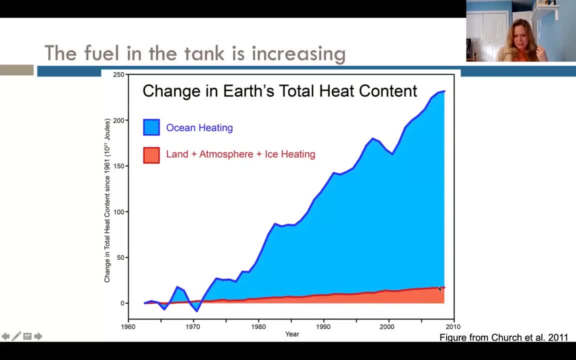 Um, the other 7% is land, atmosphere and ice heating, And so you can see these numbers there and That a jewel. so, in fact, another number that we like to talk about is That that, according to 1 estimate, the top 2000 meters of the ocean took up about 240- that a jewels of heat energy between 1955 and 2010.. 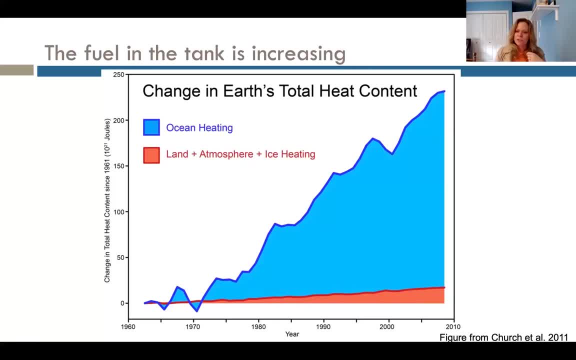 But the temperature of the ocean on average only increased by About point 1 degree Celsius, and that's of course because of the high heat capacity of Of the ocean. I do like to point out to To that it's a lower 10 kilometers of the atmosphere. We're able to absorb that same quantity of heat. 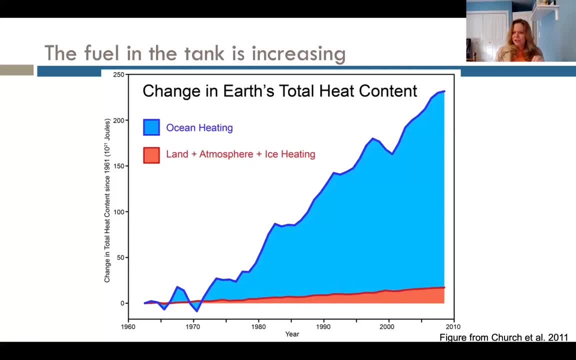 The amateur would have would have warmed by an additional 30 degrees Celsius, almost 54 degrees Fahrenheit. So in a certain sense we're fortunate that the ocean is absorbing that heat. On the other hand, if the atmosphere had warmed up by 54 degrees Fahrenheit, 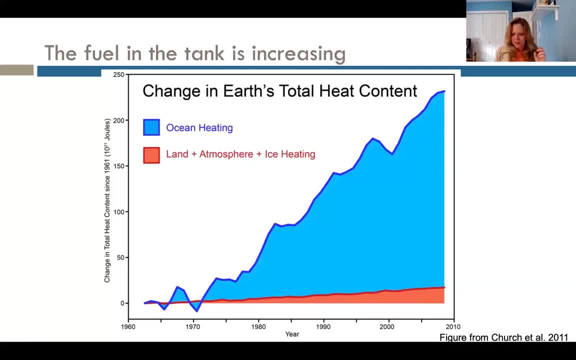 I don't think we'd be having discussions anymore about whether global work and things. So in a certain sense the ocean is kind of masking that. but The ocean is of course connected to the atmosphere and so as the ocean gains that heat, there are changes to the to the system. 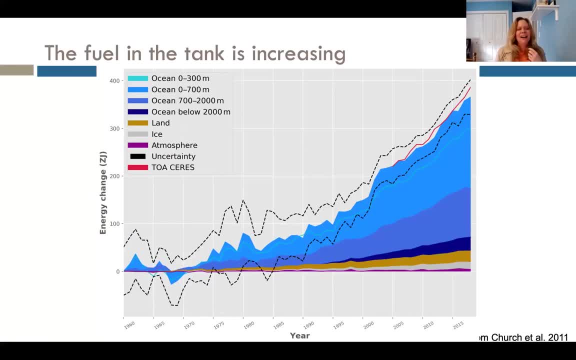 And this is just a more recent value- looking at Where the heat and the ocean is going and again now comparing to your top of the atmosphere From series, which is very similar to what we're seeing In the in the ocean heat content. so some 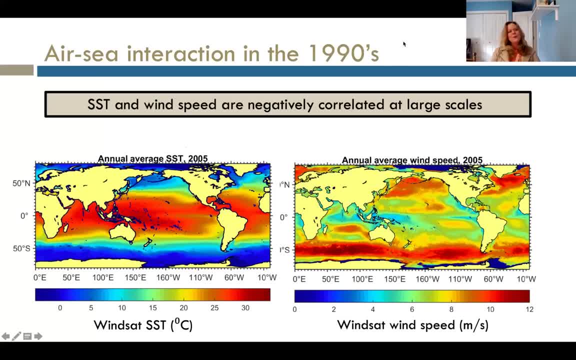 Some symmetry there. so I then like to think about what, where have we been and where are we going? And this is partially because, You know, certainly when I was in graduate school and then in my early career, sort of air sea interaction in the 1990, sort of 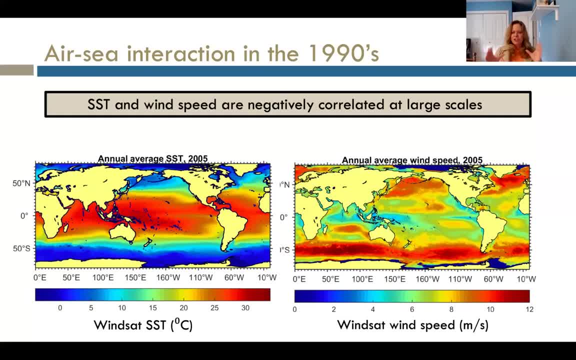 The view of this is that the ocean just kind of, You know, it moves, moves water around and heat around, but it's just sort of a big, you know Source of water and heat to the atmosphere and It's not interactive and quite the same way that you, you know, interaction was sort of like the atmosphere does things to the ocean and then the ocean just big swamp which you can take out heat and moisture from. 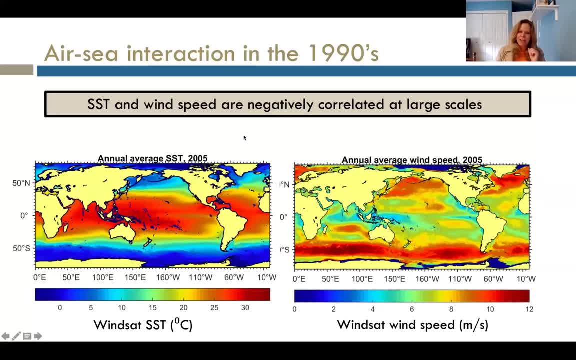 And, and to a certain extent, when you look at very large scale, that's somewhat true. So on the left is the sea surface temperature, Sort of an annual average sea surface temperature, and on the right is wind speed. And what you can see as you look at this is that 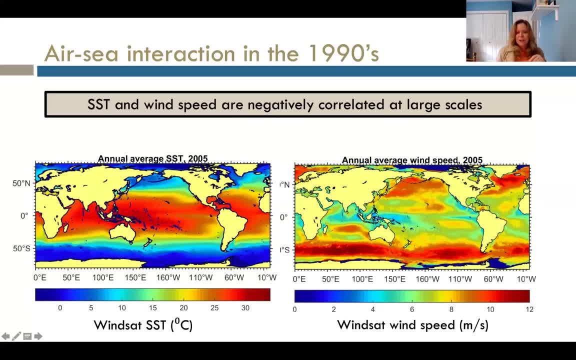 When the is high and the reds, here in the tropics, The wind speeds tend to be low, and vice versa. as you look in the Southern Ocean, for instance, you get very high wind speeds, Very, very cool, And so the sea surface temperature and wind speed. 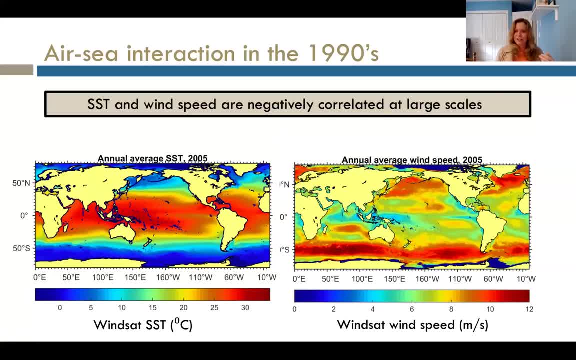 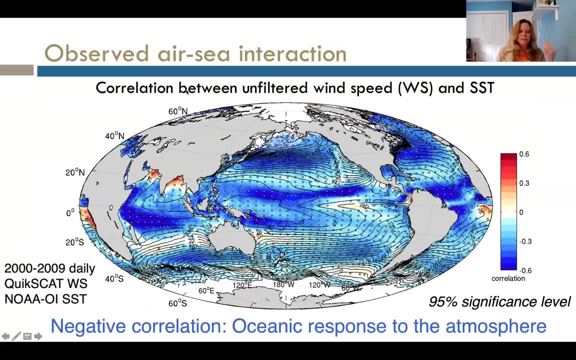 Are negatively correlated at these large scales And in fact if we do that more quantitatively, That you can see that if you just look at again it's sort of unfiltered wind speeds and sea surface temperatures And you do a correlation between them. 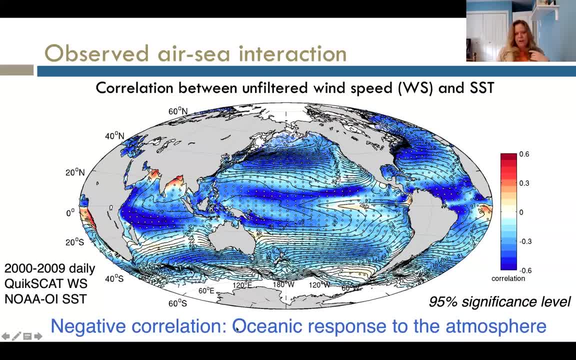 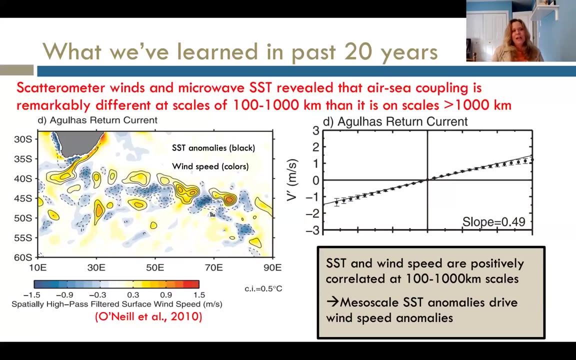 You can see that almost, almost everywhere across the ocean There's a negative correlation. In other words, The ocean is simply responding to the atmosphere, And so I would say that's you know, that's a viewpoint that is, That was quite common until about the last 20 years. So what we've learned in the last 20 years or so by using scatter on the winds and microwave surface temperature- So now we're getting down into the tens of kilometers- 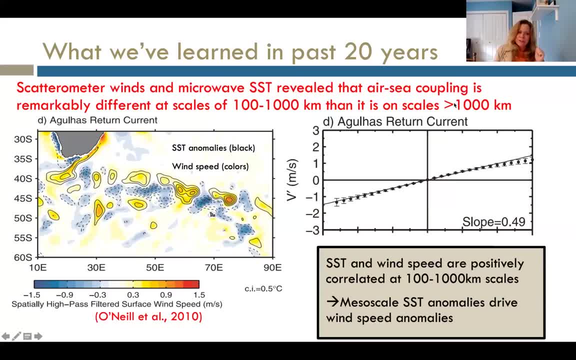 And what it's shown is that the air sea coupling is really different at scales with, say, 100 or less to 1000 kilometers. On scales greater than 1000 kilometers, If we look 1st at this figure on the left, this is from Larry O'Neill in 2010.. 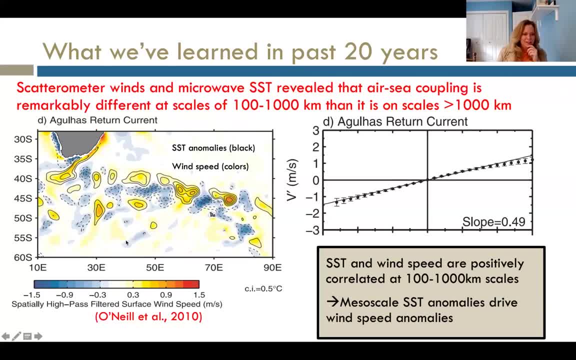 So the colors here Are the spatially high pass filtered surface wind speeds And the contours are in high pass filtered SST anomalies. so the anomalies in the contours and the wind speeds are in the colors And I think when you look at that you can see that at those scales. 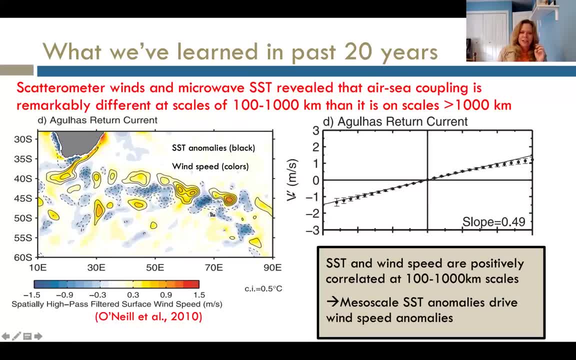 There is a strong degree of correlation and in fact That when you look at the sea surface temperature versus The anomalous versus anomalous wind speed, you get a positive correlation Between them. so the sea surface temperature would be positively correlated At these scales. what this means is that essentially, mesoscale SST anomalies are driving the wind speed anomalies. 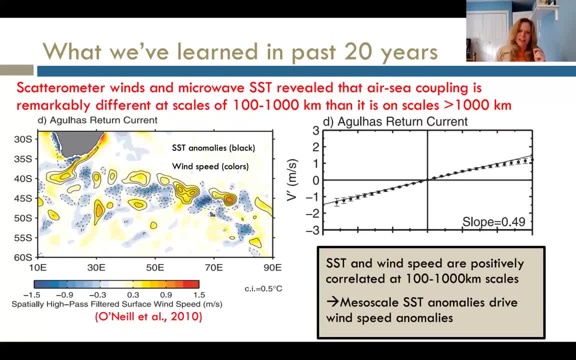 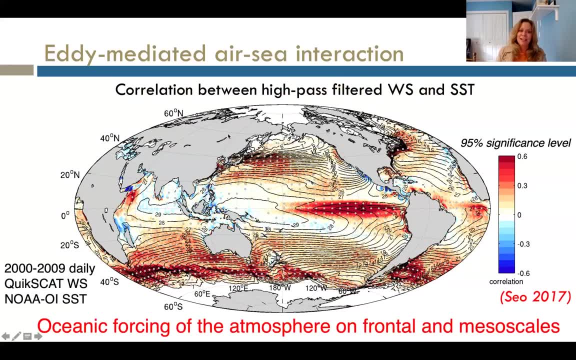 So on the large scale it's 1 picture. smaller scale Is something different. so we have now A lot of effort and work trying to understand this. Eddie mediated air sea interaction. So this is the same Figure as previously, except here we've done a global. this is here to publish this. in 2017, did a correlation between the high pass filtered wind speed and SST, So 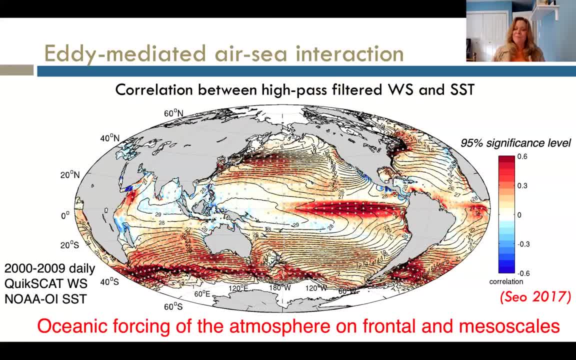 What you can see is now we have Many positive regions of correlation. So the red Is the positive correlations and that indicates regions where the ocean is forcing of the atmosphere on frontal and level scale Scales. so a little bit different picture. 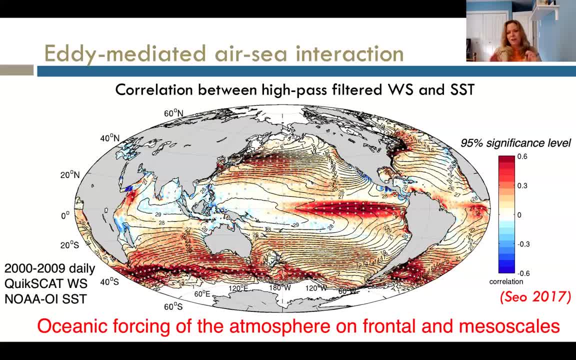 Has been emerging. so I'm going to make 1 final point about this, which is This analysis, and most of them that are done with With the data are looking at the correlations between wind speed and surface temperature, Which I'm going to show is only part of is only part of the story. So this is 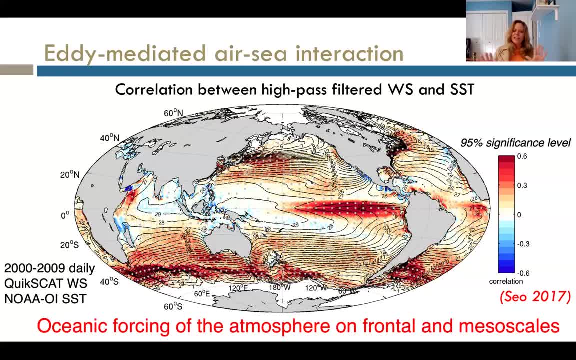 The high. if you want to think of it, we've been looking at high horizontal resolution. So as we start to look at higher and higher Spatial resolution horizontally, we begin to see this change in the correlation and how the ocean and atmosphere interact. 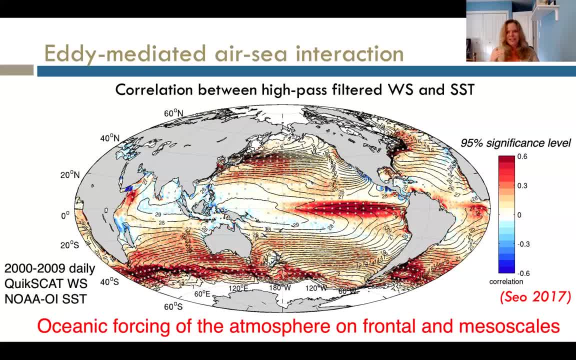 And now I'm going to take a few moments and go through Um, if we look at much higher resolution vertically, and I'll start, and I'll look for this at the ocean. So this is some work that we've been doing recently. 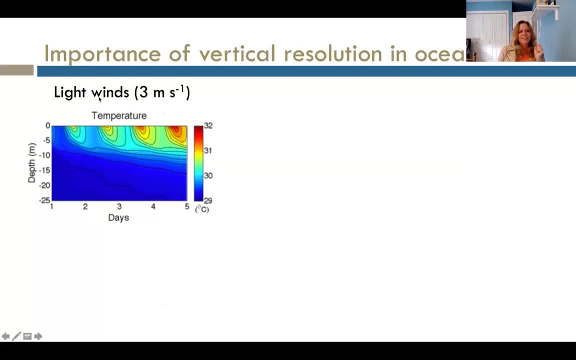 So if you look at the ocean and you're looking under conditions of very light winds, This is no model simulation in which the winds stay constant for several days, There's a solar radiation- is Is idealized. there's no rainfall. 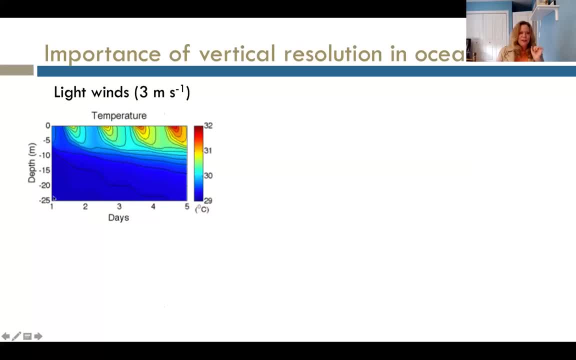 So here's depth in meters, so we're looking at just the upper 25 meters. The ocean for a few days, the colors, the temperature, Um, and what you can see every day is sort of this Cooling and then warming of the upper ocean. 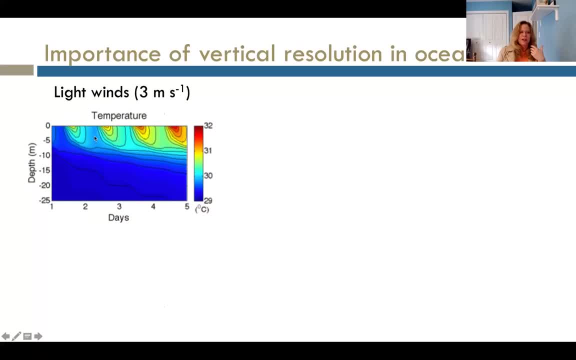 And cooling a little. at night times the wind mixes some of the cooler water up And then warming again and cooling and warming and then an overall warming trend And what you get from that. as you look at the surface temperature itself, Did you get a diagonal variability of about a degree and a half, little under a degree and a half. 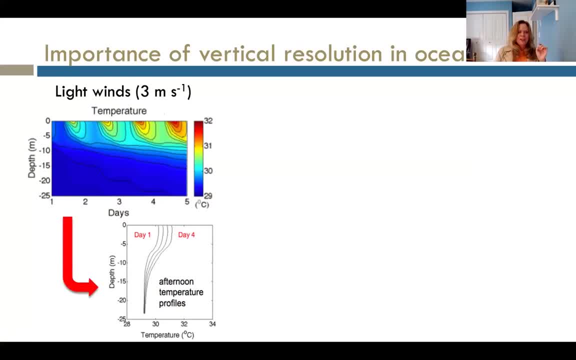 Okay, Okay, Okay, Okay. If you just look at the profiles again of temperature, so if we just take out 1 of these Time periods and take out several days every afternoon and you look up, what you can see is, you know, the upper 5 meters or so, the ocean is pretty well mixed, and then 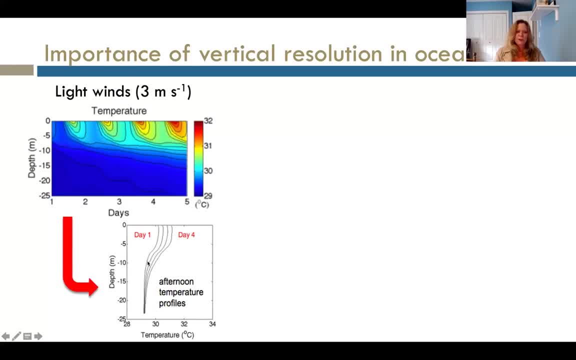 You get this, this change, down to the cooler temperature waters beneath it And then it's warming up. but you know a little bit every day And the mixing that you get from this If you look at the turbulence- kinetic energy. so how much turbulence is? 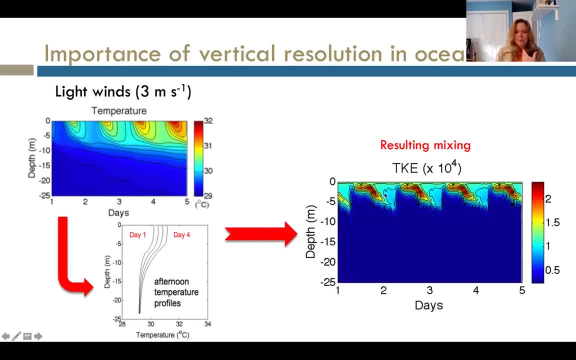 And mixing is going on in the upper part of the ocean. It's kind of, in some respects, the opposite of the temperature, when, when you get warming of that upper ocean, this is the time period where you really Cut back on the turbulence. that dies down to a large extent when the sun finally goes down and then 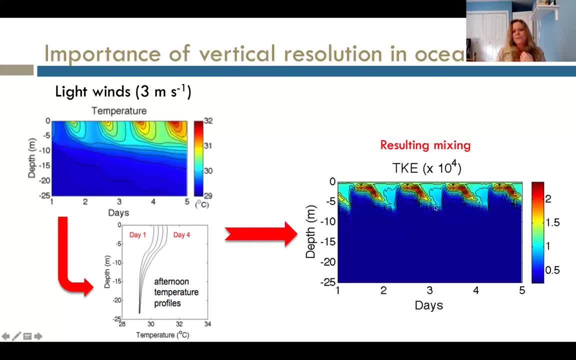 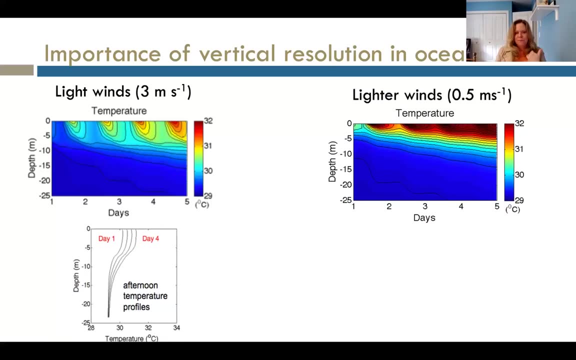 Uh, you get cooling and mixing at the surface. the sun comes up and you have just this diurnal cycle of Deeper mixing and then Um Destruction of turbulence, kinetic energy or lack of mixing As the day goes by. now what we? 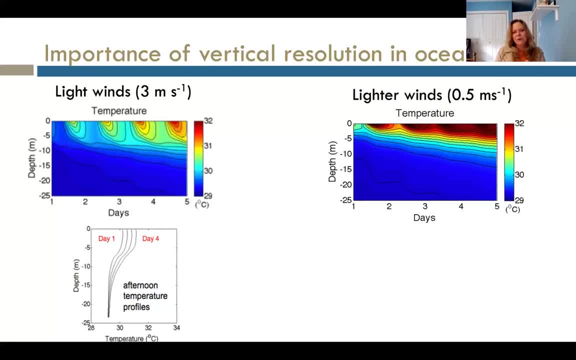 You know have had a little bit more time to look at- is what happens if you have even lighter than So. you know, half a meter per 2nd, you begin to see there's a lot less cooling During the night times and a lot more warming of the upper surface. 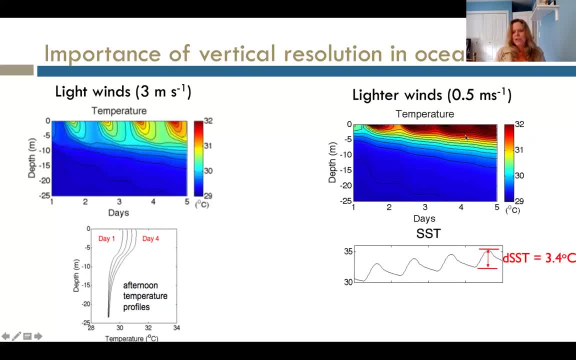 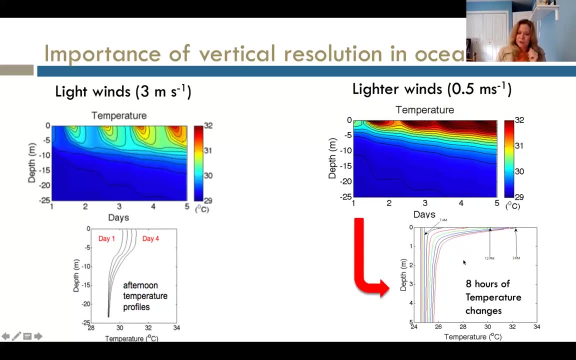 And now even more stratification. So our C surface temperature warming is now like 3 and a half degrees between what it is before the sun comes up and the peak value, And when you look at the temperatures profiles now, this is over 8 hours. 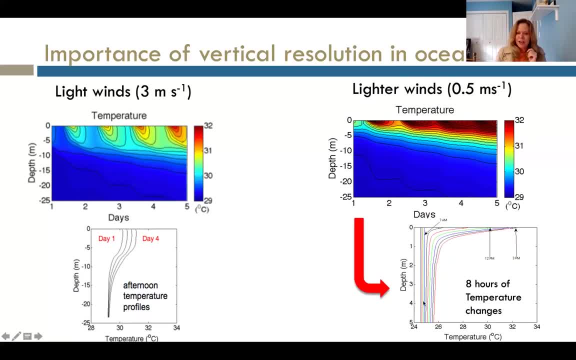 We're kind of starting off over here in the early morning And by 8 hours later is: this: is this curve here? and just to be clear now, this is that 1 meter. What you can see is that the vast majority of the change is in the upper 1 meter. 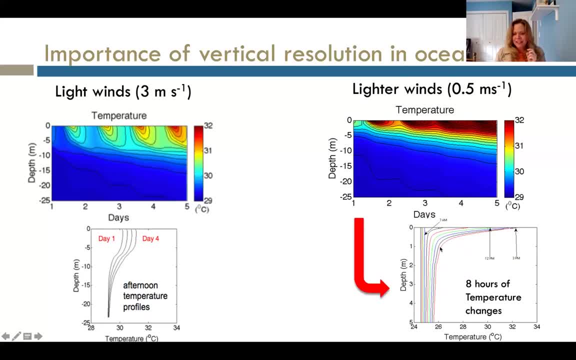 Under these conditions and this difference is Almost 6 degrees right through here, which has been seen, and we can talk about this in SS, in a satellite, SST values, but essentially What has happened is there is really no background mixing whatsoever in order to get the model to even reproduce something like what has seen of these 4,, 5 and 6 degree. 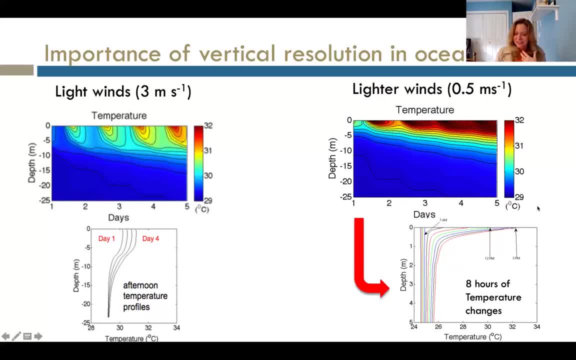 Temperatures, we have to shut basically everything off but molecular, And so the problem is is that there's no background mixing, Any more mixing than that, and it becomes very difficult to sustain this, this huge temperature change. But again, 1 of the issues is notice. there's a 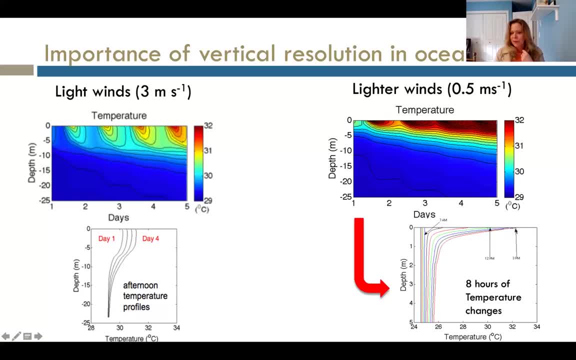 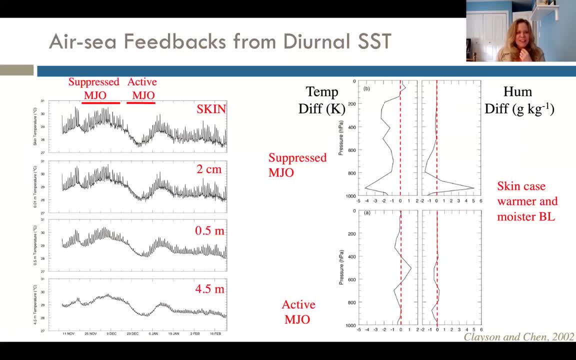 At 1 meter it's about 26 degrees, Whereas at the surface you're you're at about 32 degrees, And so that is a much more substantial difference With that. so this is some work I did a little. 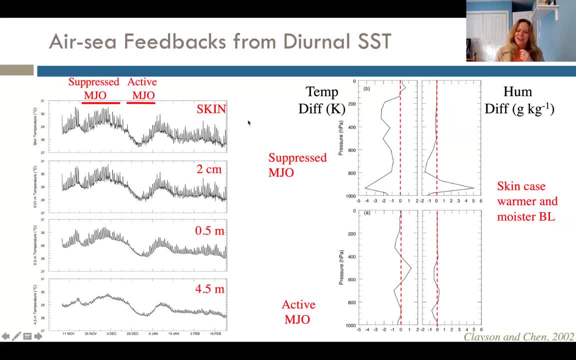 A long time ago. as it turns out now, this is now what I did. from this: 1 is I use a couple Single column model set up for the toga core, So tropical Western Pacific Time period. so I had a high resolution ocean running under the 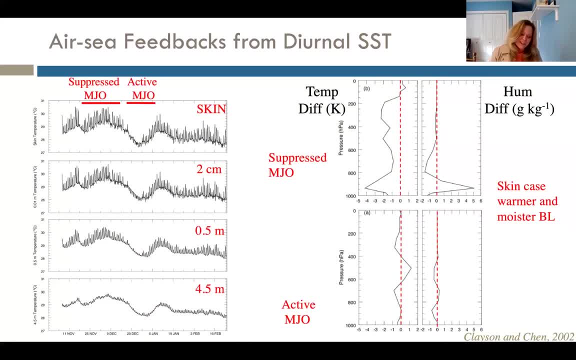 The end car, the scam model, as a single column atmospheric model at the time. And what? what I did for For this series of experiments is that I chose the depth Of the ocean to, to basically to tell the atmosphere, to, to give to the flux parameterization so that the long way flux and the latent heat flux and the sensible heat flux. 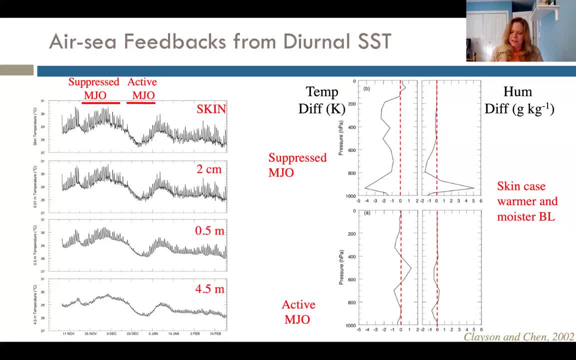 We're using a value at a depth that I prescribed. So, if we look to the last here, so this is a 4 month, the 4 month intensive observation observations period of toga core. So this is C Surface temperature, and so you know, every day we see these. 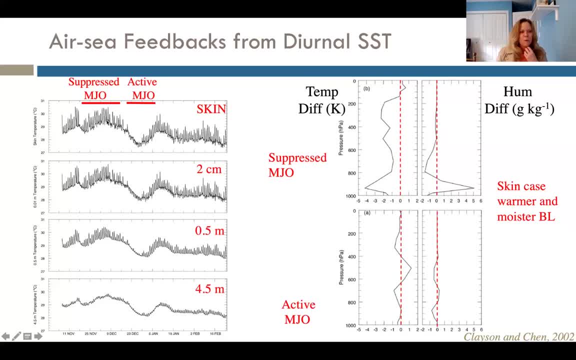 These, you know, nice strong diurnal warming, This time period here with during the suppressed phase of the Madden Julian oscillation, which is a 30 to 90 day oscillation that propagates through the topic and becomes coupled with convection over somewhere over the Indian Ocean. 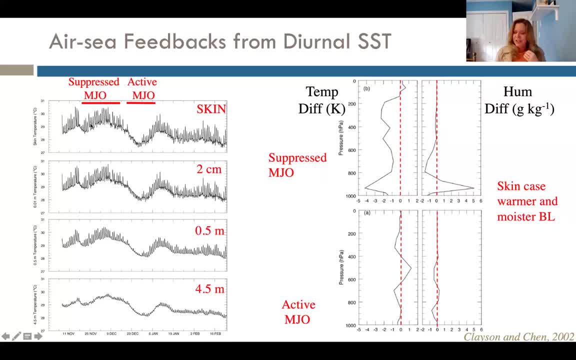 And typically during these suppressed conditions it's sunny, the Windsor, the Windsor Light, followed by an active phase of the Madden Julian oscillation in which it was The winds were much higher, it was cloudy storms, And so what you can see during the suppressed conditions are, as you might imagine, low winds and high solar insulation, So lots of darling warming. 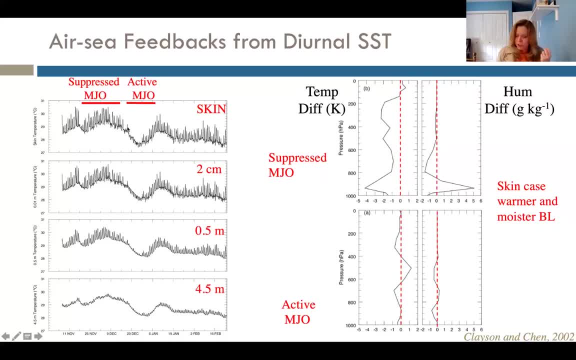 Then, when the active phase starts out, you get, get cooling of the. you see very few days with that diurnal warming- And then, once it starts to pick up again- this uppermost plot is the skin- And then, once it ends, it starts to pick up again. 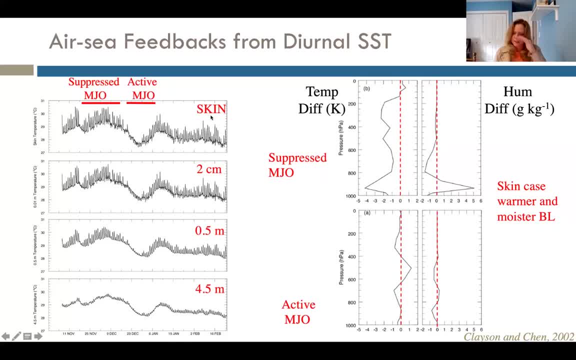 This upper most plot is the skin Value, which means you know, really, our best estimate of that true interfacial Temperature. this next spot is at 2 centimeters In the ocean, for reasons we won't talk about too much here, but for those of you who are very fond of the skin, 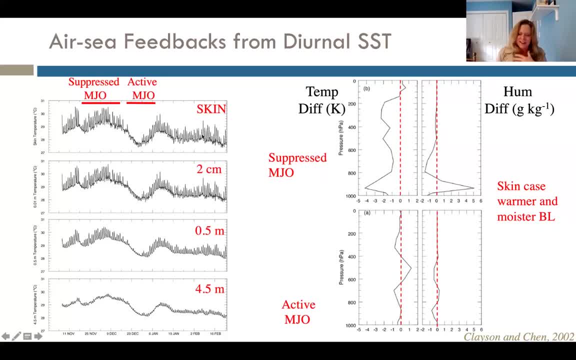 The cool skin effect that the skin is often about 2 10th of a degree cooler than just beneath the skin. So there's about a 2 10th of a degree difference between these 2.. As we go down a little further in the water column- this is about half a meter down and 1 can begin to see a reduction in that diurnal warming during the suppressed phase. and at 4 and a half meters, which was the depth of many of the measurements during to the core. 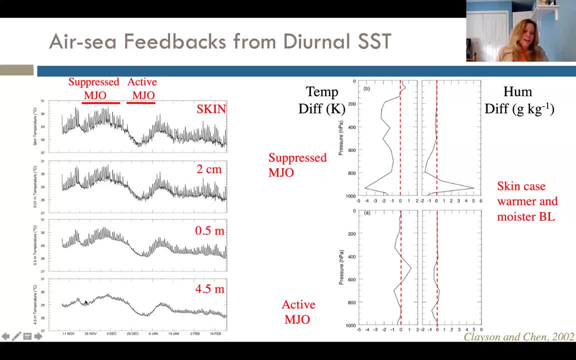 There's very little in the way of diurnal variability. So I then took the basic run and, instead of coupling the skin to the atmosphere, Couples the core and the diurnal. So I then, So I then The 4 and a half meter temperature to the atmosphere allow the models. the models all run the same way. The differences in what temperature. I was getting to this And I was thinking I might see some differences. 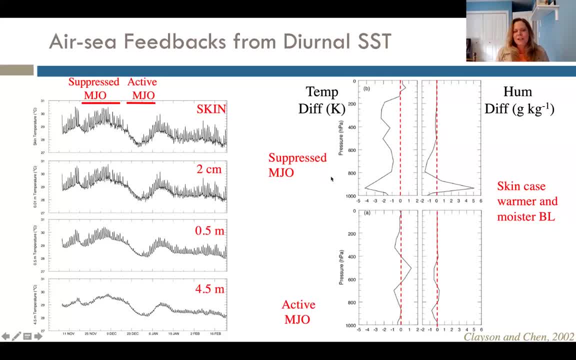 So in the but I was a little surprised to the differences I saw. this is the suppressed Time period. the bottom 2 plots are the active time. On the left are the temperature differences And on the right are the humidity differences. 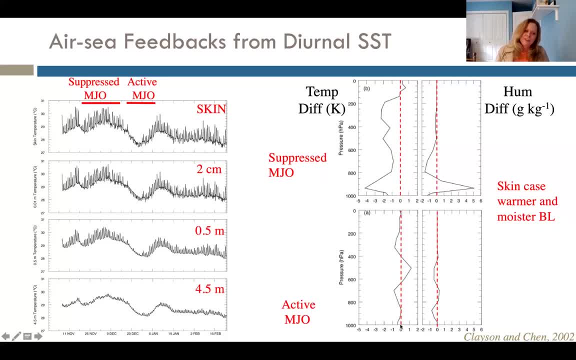 So very few differences Between coupling with the skin or the 4 and a half meter During the active, because they're not wildly dissimilar from each other. But when you look at the suppressed, what you can see is that these are now. 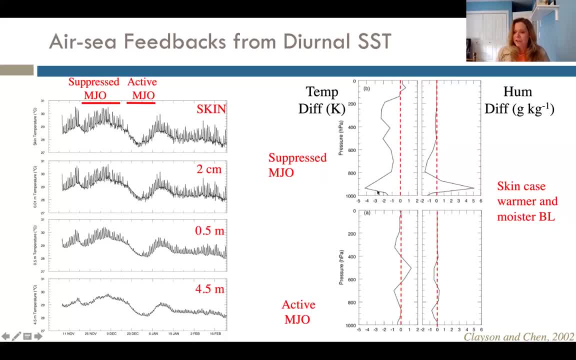 Up to 4, and this is now the mean during the entire suppressed phase. the difference, You see, that the skin case results in a much warmer and more voice Atmospheric boundary layer and that, in fact. there you see the ramifications. 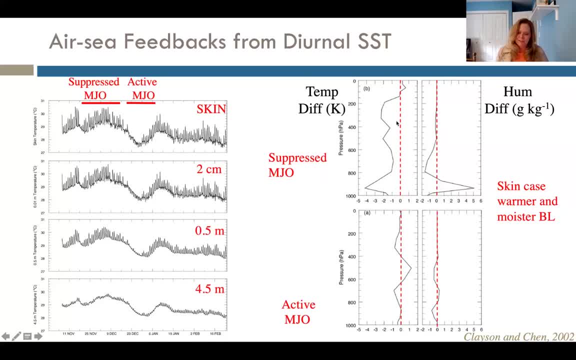 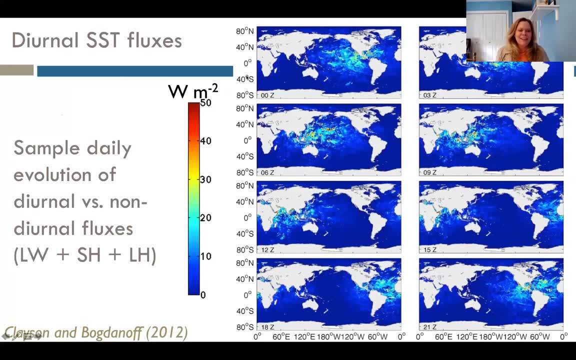 Of that kind of up through the column itself. So if we look at the diurnal impact of fst flexes, This is just if you allow the ocean to warm During the day and calculate the flexes, versus if you sort of artificially keep it at the nighttime value, and this is 0, Z to 3, Z to 60, so forth, every 3 hours. you can just see. 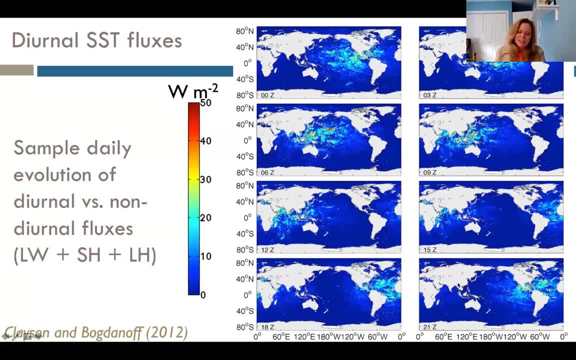 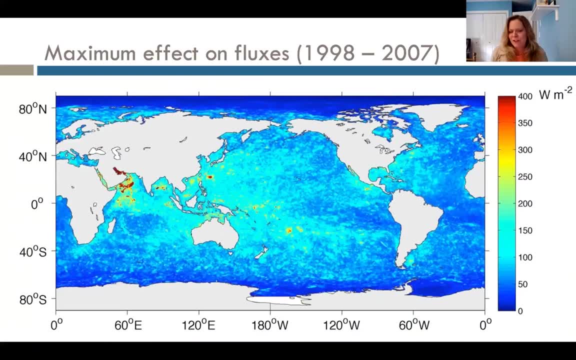 The progression of the warming from the, The sun and you see aspects of winds picking up and so forth. If you just go through, this is now using the satellite data, And if we just take 10 years of it and say in those 10 years, at any given spot, what was the biggest difference between including the diurnal warming and not? 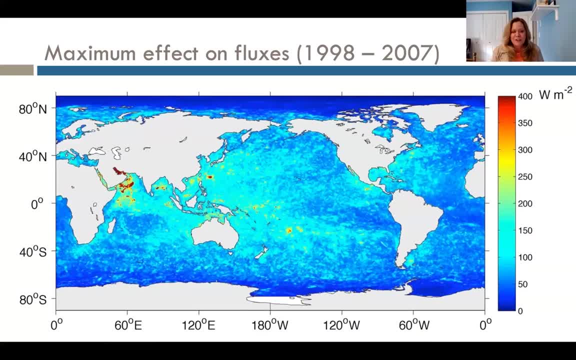 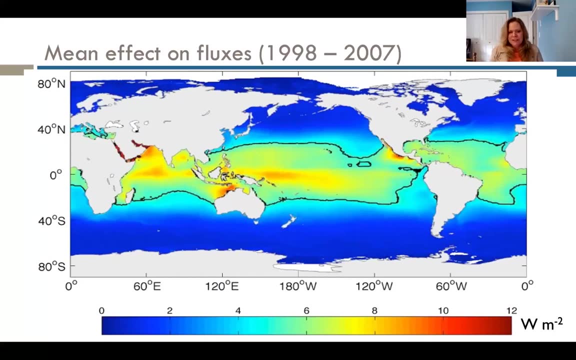 This is what you see, so you can see values where it's 200, 300. And up to 400 watts per meter squared difference, using that title and then not including that And the mean effect on flexes then. so over 10 years, all time periods. 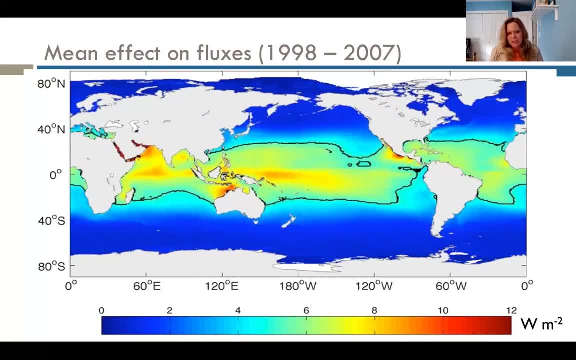 It's, you know, it's, it's, it's you know, 5 degrees globally and it's over 5 degrees in the in this topic. So when you're trying to get a balance, This turns out to be important. but salinity also stratifies the upper ocean. 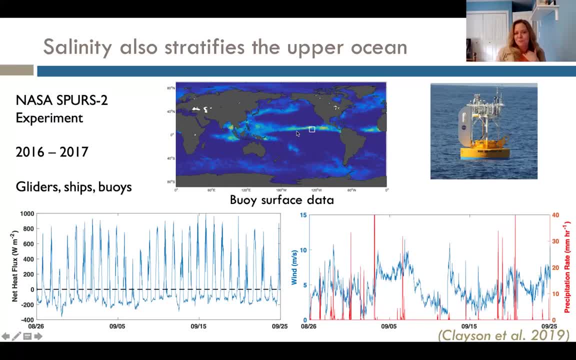 So this was data now from the NASA Spurs to experiment which was located. this box here is basically where the Ship was and there was a buoy in the center of it and it's really in the in the Eastern tropical Pacific. Um, here's just some data from the buoy. 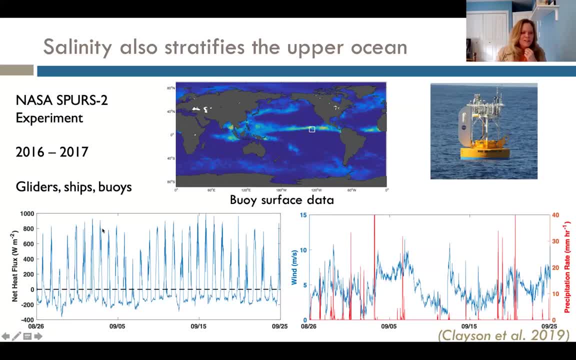 You know, here's the heat flux. so daytime peaks, solar radiation, night time Loss of heating by the ocean, wind speed. here on the right and the blue, we had conditions of up to about 10 meters per 2nd, but we also had days where it really was about 1 meter per 2nd. 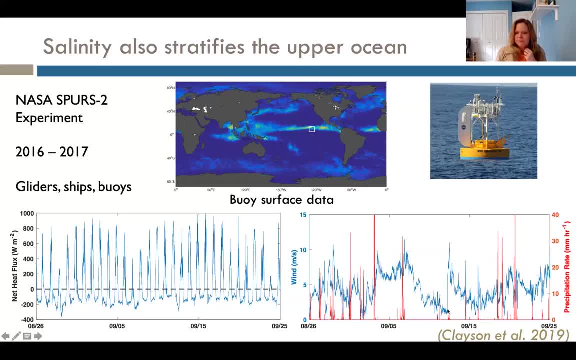 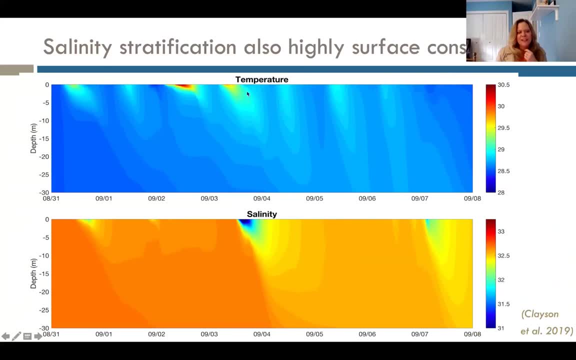 Um, and the red is just sort of the, the rain that was just episodic throughout this time period. So, if you look, this is somewhat analogous to the figure that I showed before, but using the real data, And so this is the temperature and you can see sort of the daytime warming and that real stratification again, and just the upper. 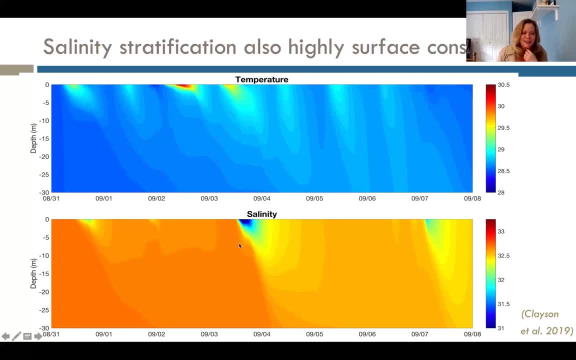 Meter. but you can also see that the impact that a salinity rain event has. you can see just that, the freshening of the ocean, a little bit of freshening. This was a large freshening event and again, a large difference in just the upper few meters. 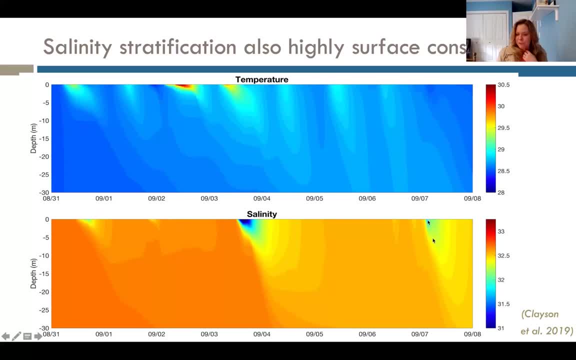 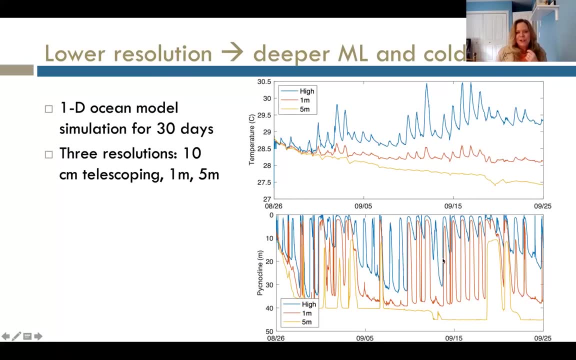 There's another series of rain events towards the end of that time period, but the rain, the winds are much higher, So there's a lot more mixing through the ocean column. So, given that there's so much variability in the upper part of the ocean, we thought let's let's explore how important that resolution is on the ocean side. 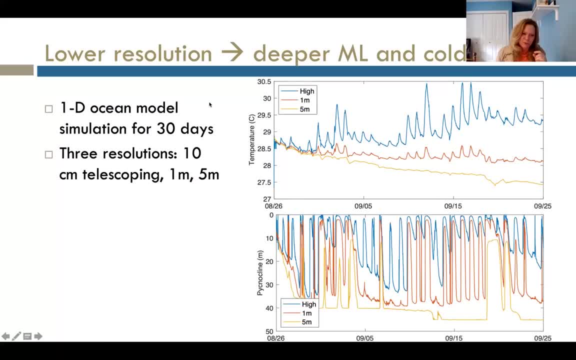 So what? what we've done here is I've run a 1 dimensional ocean model simulation For 30 days and we're just looking at there's- there's no coupling. We're just looking at. if you had the same heat fluxes coming in but you had different vertical resolutions of the ocean mix layer model, What would you see? So we had 3 resolutions. 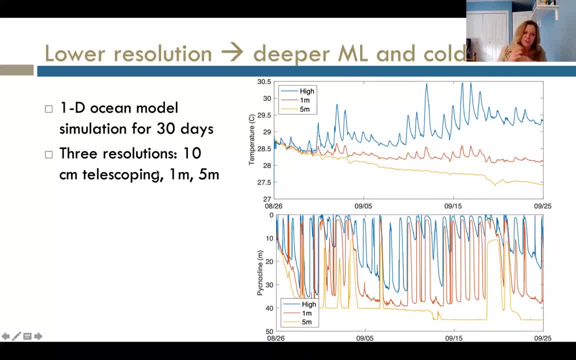 With the 10 centimeter telescoping resolution, which I'll call high resolution here. Then I had it at 1 meter and I had it at 5 meters And what you can see is the difference between the blue is the high resolution. 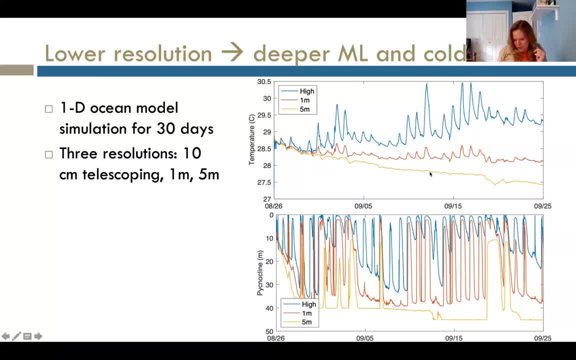 The 1 meter And the 5 meter resolution and you can just see that the cooling that is different, even on the. you know the long term trend between the high resolution, the 1 meter, even the 1 meter and the 5 meter. 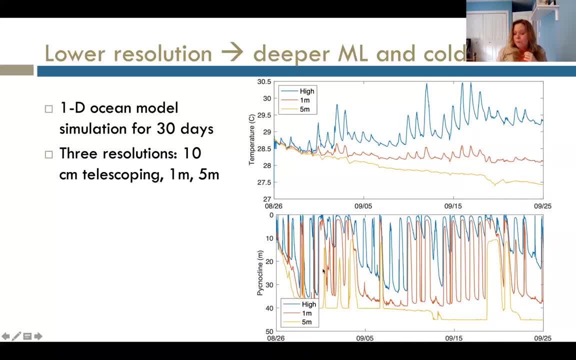 Down below, here is the depth of the picnic line, essentially the depth of the mix layer, And the blue again is the high resolution. What you can see is just that, Even even with a 1 meter resolution, We're not- you're not- constraining that heating. 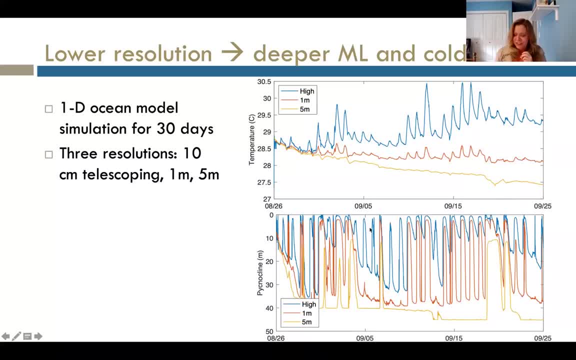 Right into the upper part of the ocean. nor are you constraining that freshening That's also contributing buoyancy to the upper part of the ocean, And so when you don't resolve that, you get mixing much deeper and that causes colder. 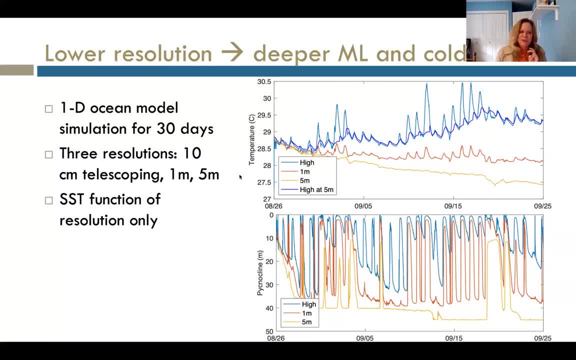 And just to demonstrate that the future of the center is a function of resolution only, If I take the high resolution model run And I just pull out the value at 5 meters from the high resolution run, That's this blue, This darker blue line, which looks exactly like what we expect to see. So it's not the fact that I'm just looking deeper at this 5 meter. 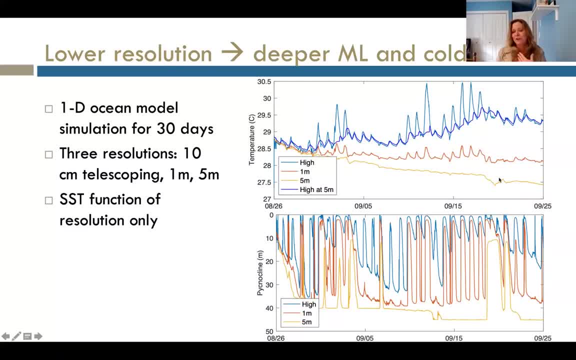 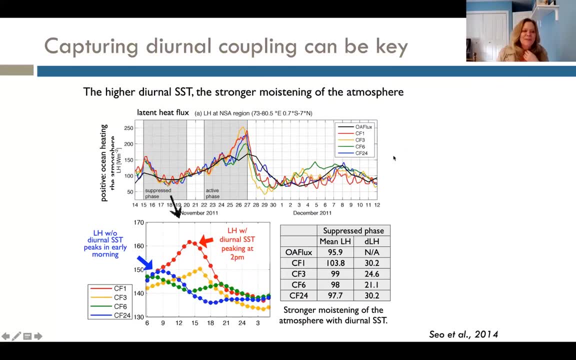 Value. it's the fact that the resolution is different and we're not really trapping that stratification near the circle. So this is again work by And which he was looking at, the with a, with a coupled model, And basically showing that when you couple the model more often 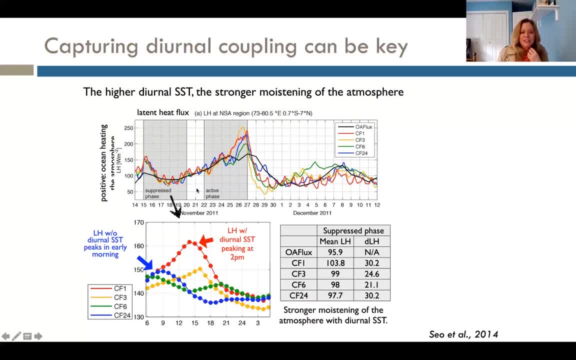 So you're, you're capturing the dinal, you get more moistening of the atmosphere And you have a different timing of your peaks Of of when you're late and he flex is the strongest. So when you have the dinal, SST that peaks at about 2 PM and is stronger. 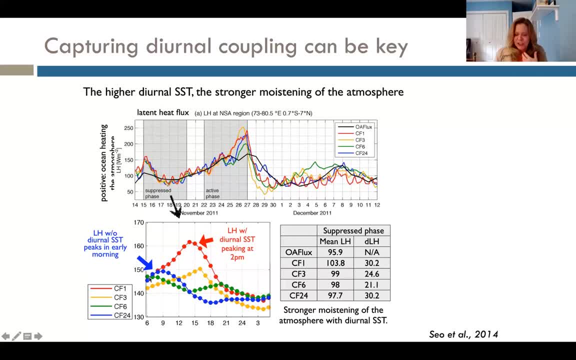 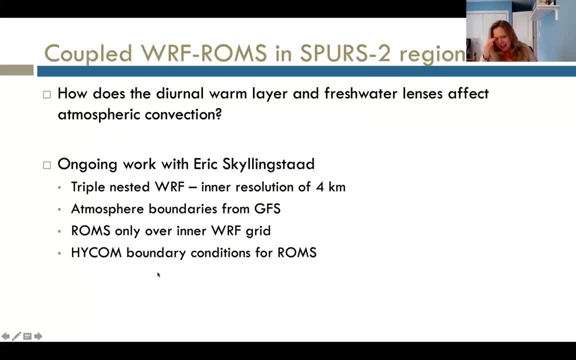 Then when it, then when you are coupling the ocean atmosphere, so once every 24 hours And it's much less so. this is some work now that I've been doing with Eric filling sad And we've been really trying to ask ourselves: does any of this matter in the long run, these kind of small variations here? 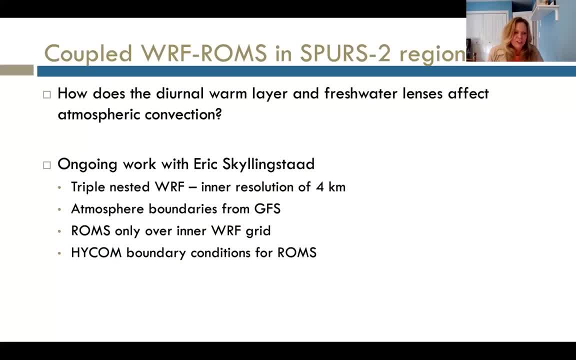 And so we've run a couple of war from simulation. So the horizontal resolution is about 4 kilometers And the we're running ROMs for the ocean model underneath war And what we, because of constraints computationally, We have 2 simulations here that I'm going to show you. 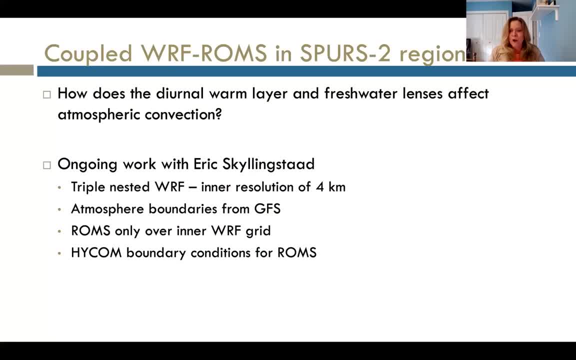 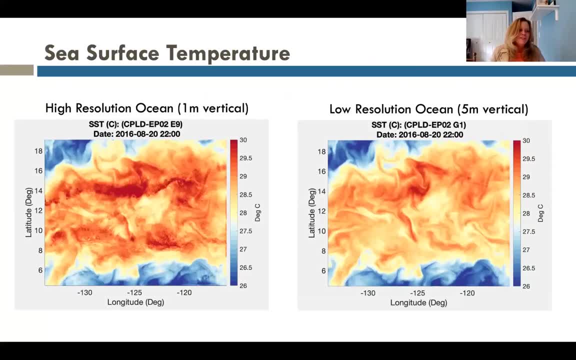 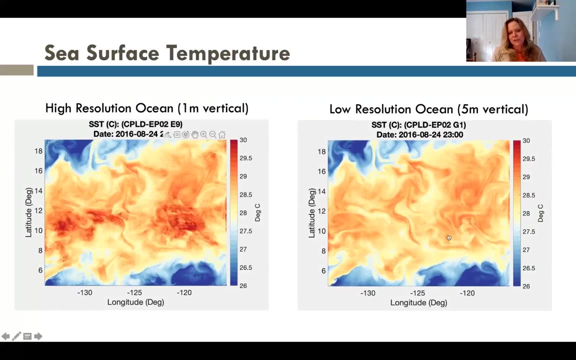 And 1 of them we call the high resolution, but I will emphasize is that 1 meter vertical resolution and low resolution, which is a 5 meters Resolution. so this is the sea surface temperature from those 2 simulations. So the higher resolution results are on the left and the low resolution results are on the right. 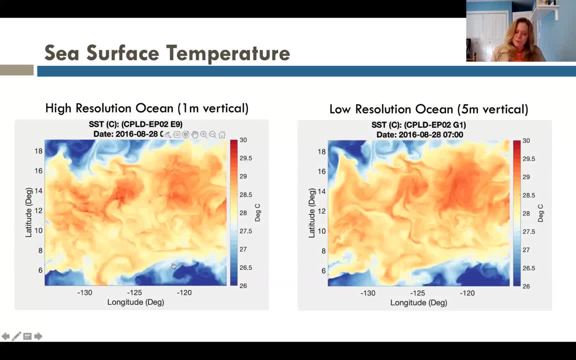 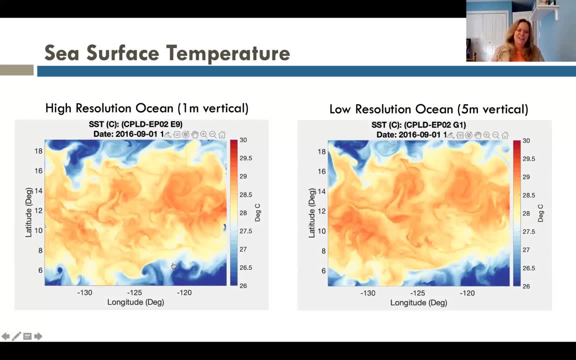 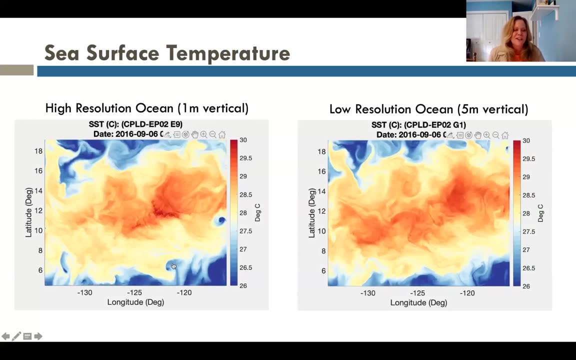 1 thing that you can definitely see is how much more diurnal warming there is On the in the higher resolution ocean simulation I like to think of. This is the lungs the ocean looks like. you can see the ocean breathing and you can see it's breathing so much better when you have a little bit higher resolution and really capturing now what's happening. 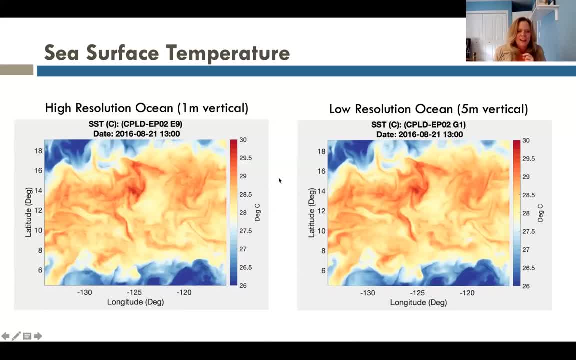 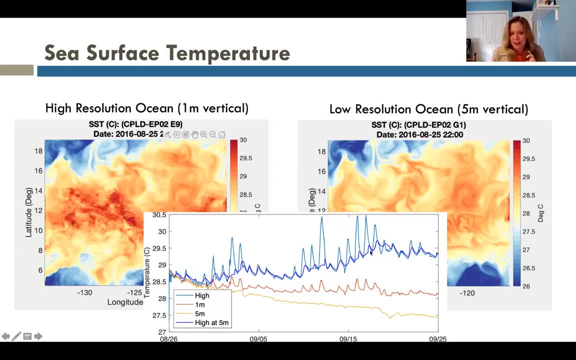 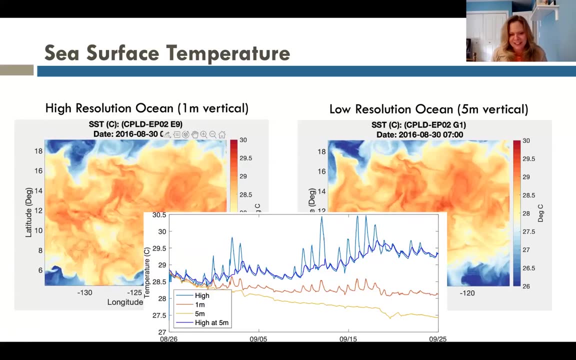 At the upper, at the upper ocean. and then, just to emphasize, this is now a 1 meter vertical resolution and a 5 meter vertical resolution. We're not at a high high Our resolution for the ocean model. right now we're coupling the cloud. 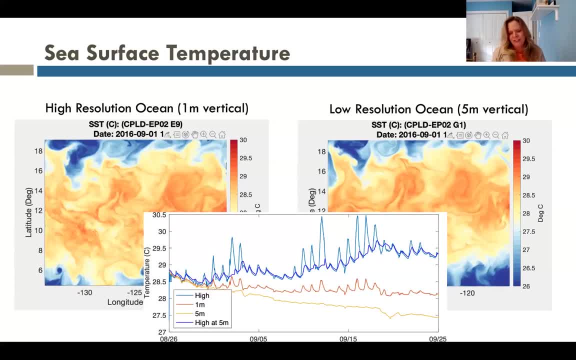 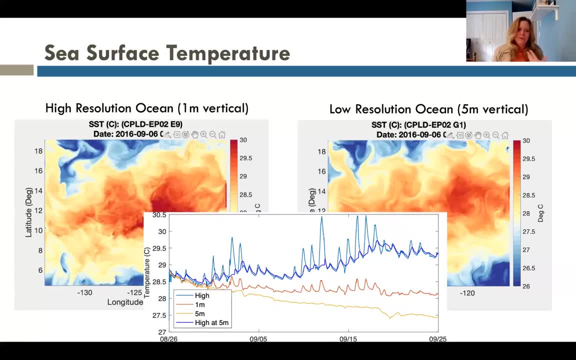 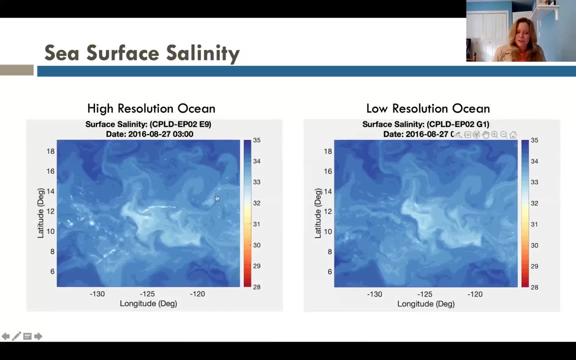 To a series of 1 dimensional high resolution ocean 1 D models to to Try to address. try to address it with: We had a higher ocean resolution. This is now the same thing but surface salinity. so again, the high resolution option on the left and the low resolution on the right. 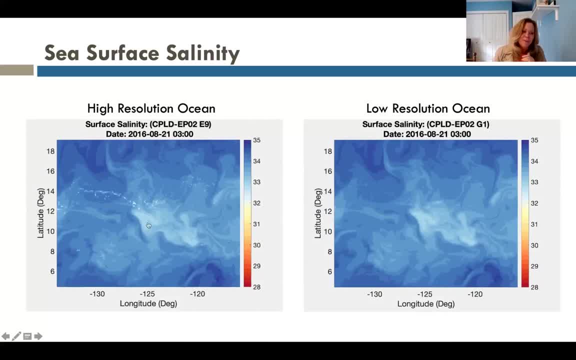 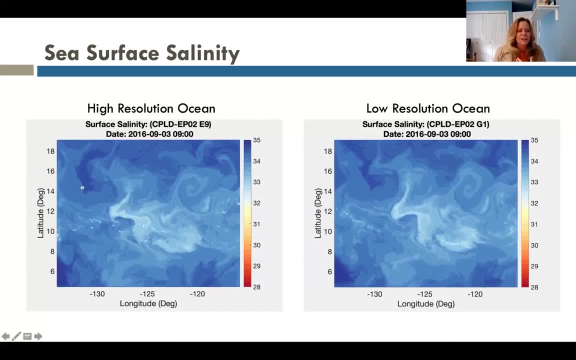 And so, just as you watch, again in time, you can see a lot more of the fresh water lenses. or: Yeah, yeah, Yeah, yeah, yeah, no, that's impressive pools of fresh water. um, under the under the higher resolution, because again it's doing a better job. 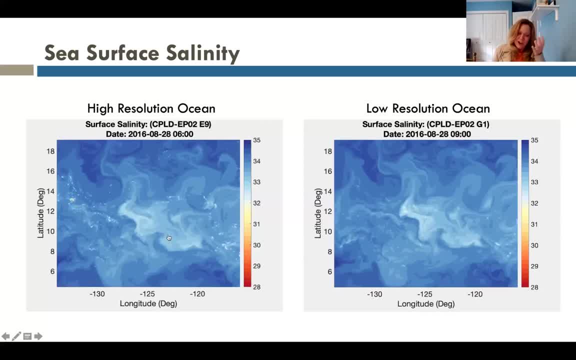 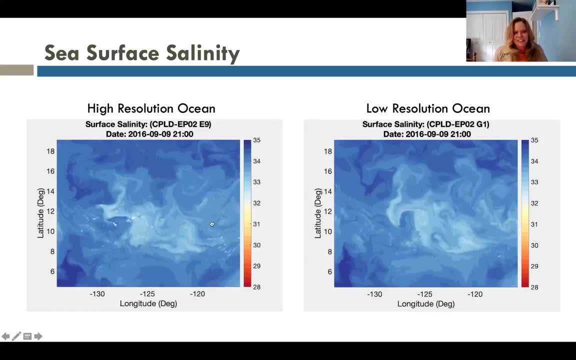 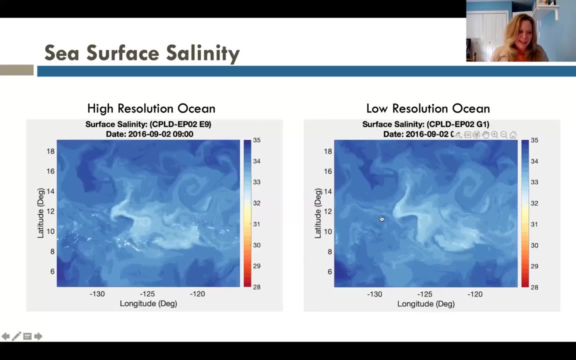 of capturing the fact that those are sitting at the top of the ocean and they're they're not being mixed down through the upper five meters right away, and so you can just see the difference in the in the number and strength of those pretty small scale rain events and their impact on the ocean. 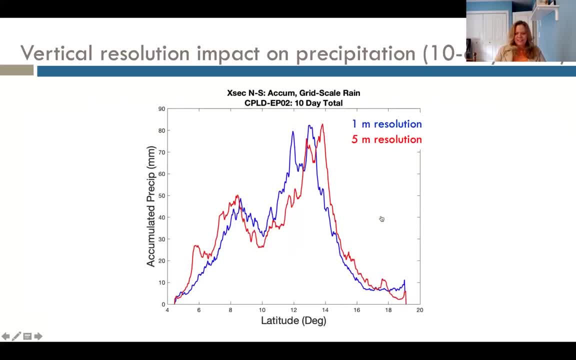 so the question that we should should ask ourselves, then, is: what impact does that have on precipitation? and this is one of our initial steps on this um is to look at the impact on the precipitation. here's a 10-day mean, and this is the accumulated precipitation. the blue is the one. 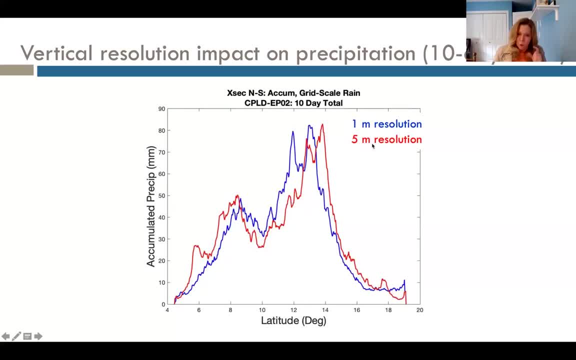 meter resolution model and again, that difference in resolution is only in the ocean. so it's with a one meter ocean resolution or a five meter ocean revolution, and this is now zonally average. so latitudes here, um, and what you can see is that you know in after about 10. 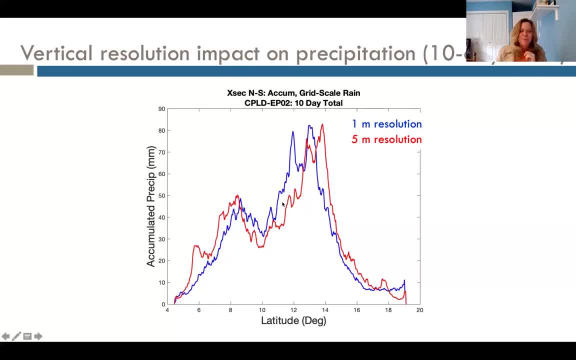 days that accumulated precipitation sort of that, the peaks um are actually shifted away from, you know, away from the center of the domain in the five meter resolution compared to the one meter resolution. so even even impacting even that little bit of difference that we're seeing between the 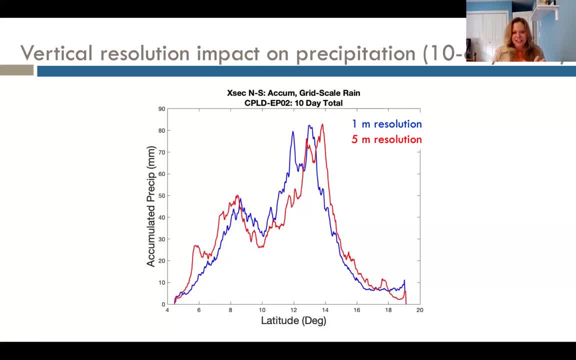 the warming and the freshening. when we couple that together, we're seeing differences in the convection and the precipitation field. so i've been talking a lot about vertical resolution. i'm going to switch back now to horizontal resolution, because one of the things that we are very 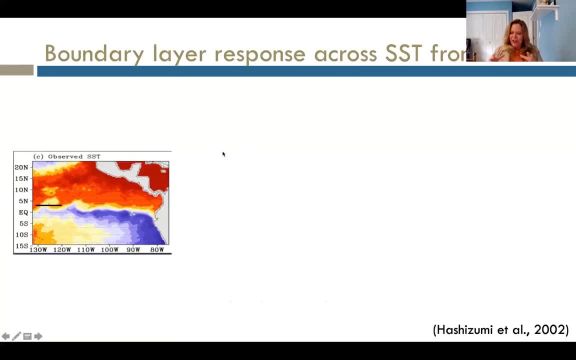 interested in is how, how is it, you know, how does the coupled system sort of respond now vertically? we realize we need to know very um, we need to know what's happening there. we also need to know across the surface temperature front. so this is now the tropical eastern pacific, not too far from where this first tuesday was. 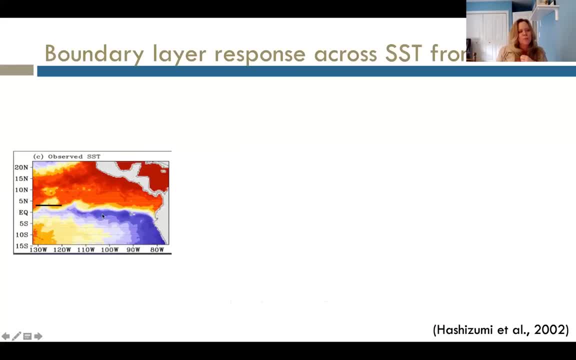 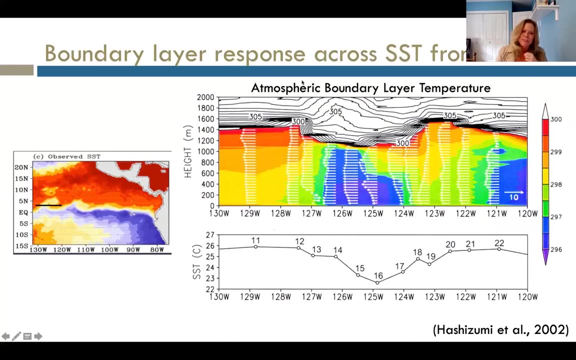 we have these. uh, this is sea surface temperature, so the cooler water in the blue, warmer water in the red, and there was a ship track um that that went across, sort of so warm to cold to warm um, and looked at now this is the atmospheric boundary layer temperature and down. 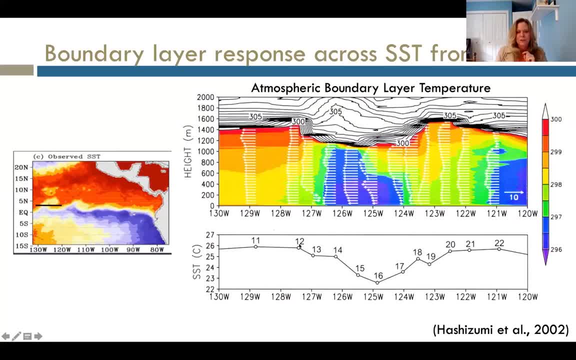 is the sst, so you can see that you know as it. as we're looking at the depth of the mixing and so forth, you can see that change in the atmospheric boundary layer that goes across this as you look, uh, over the colder water versus the warm water. so to explore that a little bit, there was an 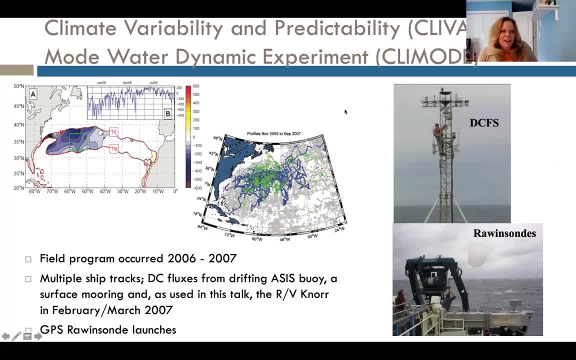 experiment called the climb. it's called climode, which was the clivar variability and predictability mode water dynamic experiment in the gulf stream. it occurred in 2006 and 2007.. um, it was really designed to understand mode water formation. so there were. 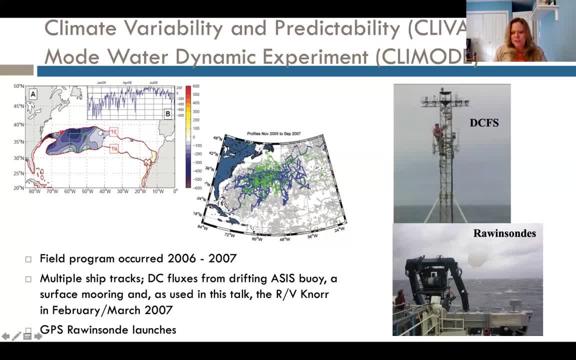 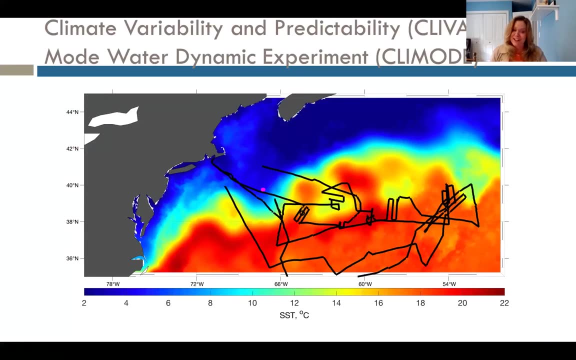 some measurements of fluxes and some raywin songs were launched um from this and so, um, we can do a little bit of work. now i like to show this figure. this is what happens when you let the oceanographers drive the ship um, so you get this kind of a ship track which makes sort of interpreting things a. 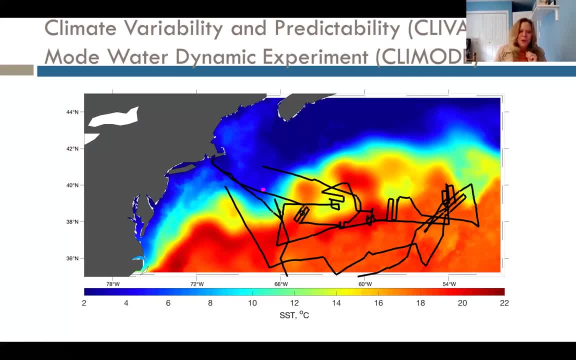 little bit, a little bit difficult, but we're going to pull just a little bit more of this, just one, one component of it, which is really just this ship track right here, the sea surface temperature in the background, um, so you're going to see across in the top part here where the ship. 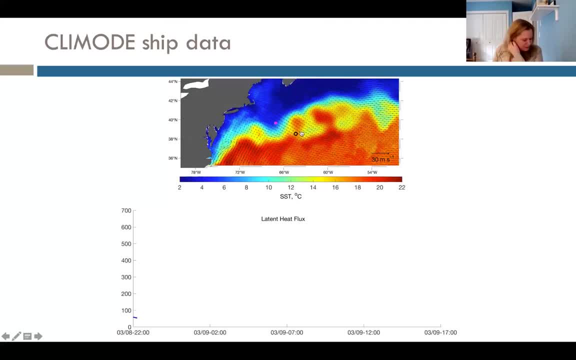 we start at the pink dot, the uh, the circle. here is where the buoy is, so we're going to see the ship moving across. the bottom figure you're going to see is the latent heat flux, and it goes from zero to 700 watts per meter squared. 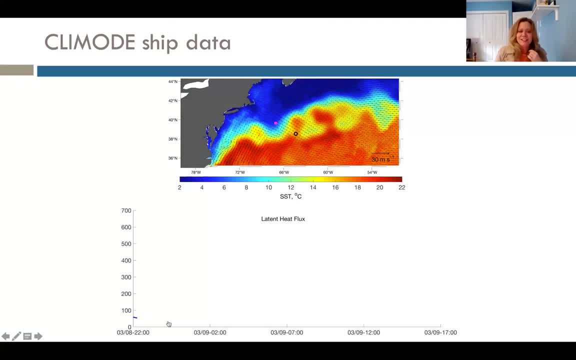 uh, in the value you will see a color. the color of the line is the sea surface temperature is measured by the ship. so you can see as this is going. so the cooler water, um, then it warms up a bit. we get higher fluxes, warms up again, stays pretty constant, um, and then we hit some warmer water. 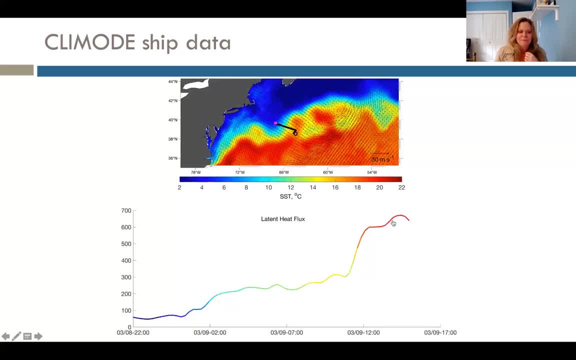 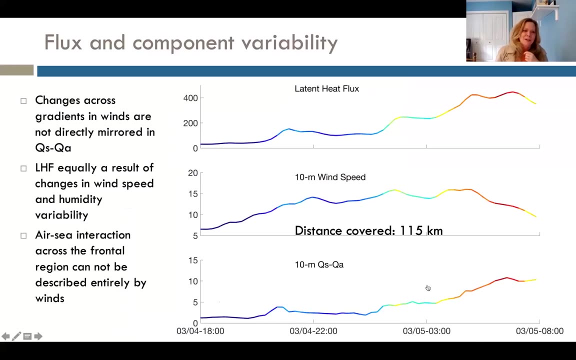 and really warmer water and we we jump up to, uh, almost well over 600 watts per meter squared, which the change can be as much as 300 watts per meter squared in 19 kilometers um. so one of the reasons that i want to point this out is that if we take sort of a similar ship track, when we have lots of data, and look at that, 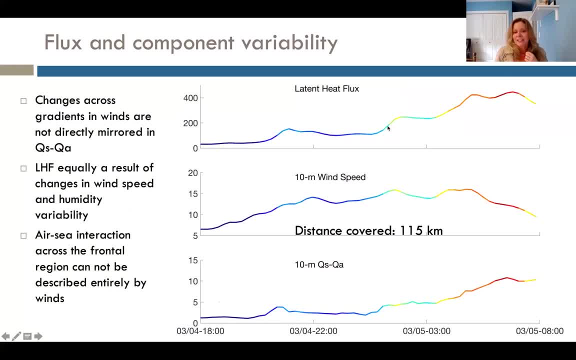 here's the latent heat flux change. so again the color is the sea surface temperature. in all three of these plots this is the change in latent heat flux over the track. This whole track here is about 115 kilometers. Here's the change in the wind speed. 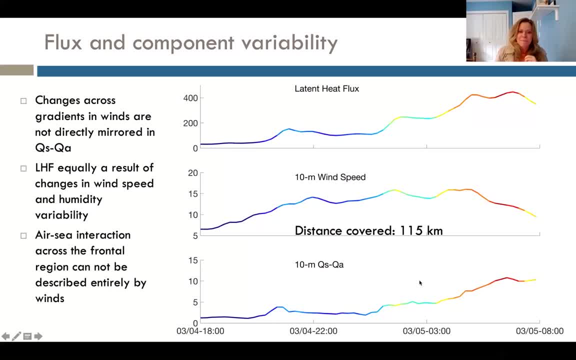 You can see, as it gets over the warmer water it decreases. So this increase here in the latent heat flux is actually caused by the change in humidity difference between the ocean and the atmosphere. So one of the reasons that I point this out is that much of our work on understanding 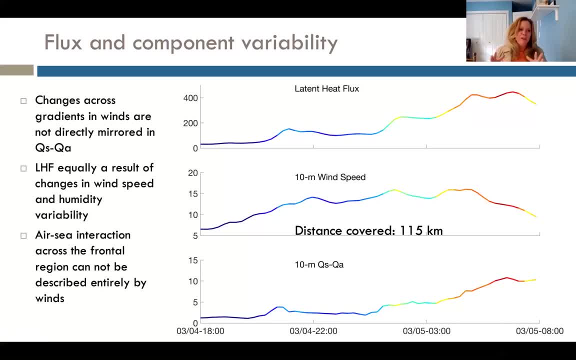 sort of the horizontal impact variability has been looking at wind speed and sea surface temperatures, But we're only capturing some of the interactions by that. That air-sea interaction really cannot be described entirely by the wind And you can just see the differences in fluxes. 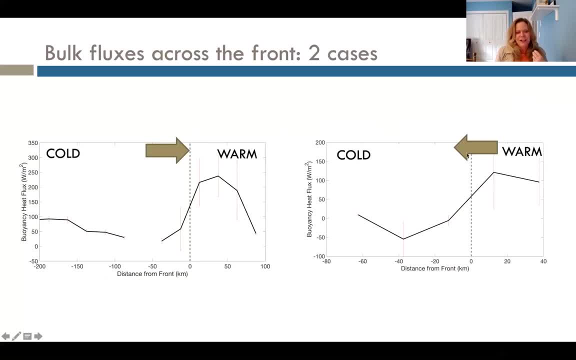 here. So this is distance from the front. The fronts are here. I just want to emphasize what I was showing. there was a case of cold air flowing across warm water, So low latent heat, buoyancy fluxes and then higher If you go from warm to cold. 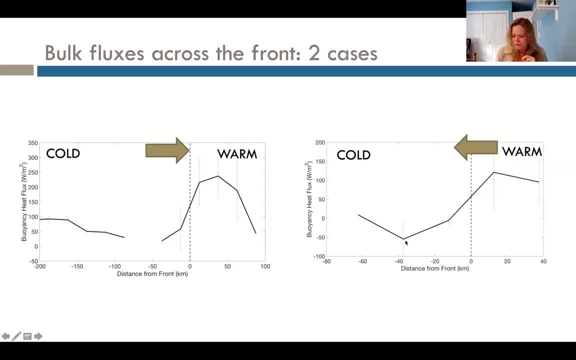 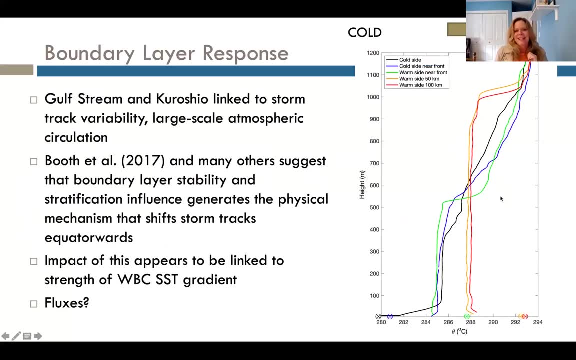 the magnitude is much less And it actually goes negative here as you're working to stratify the upper, the lower atmosphere And this is again a cold to warm. Now we're looking at the ray-wind song And you can hear: 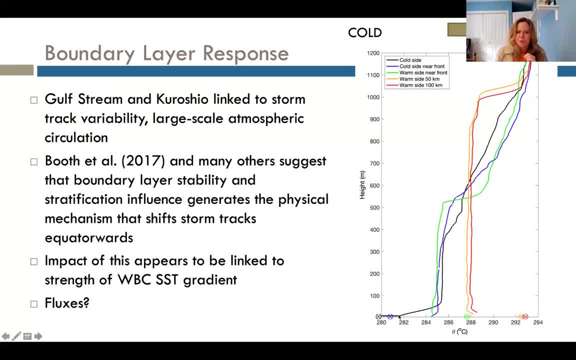 So black here is on the cold side, Then blue is we're getting closer to the front. The dots here are sea surface Temperature. So you can see the change even in that from here to here, in just that last little surface layer, just before the ray-wind funds pick it up, And then the warming of the you know. 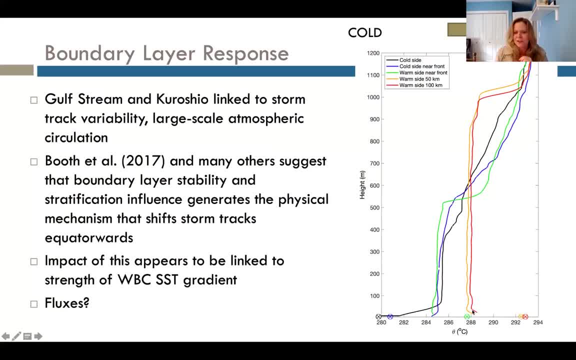 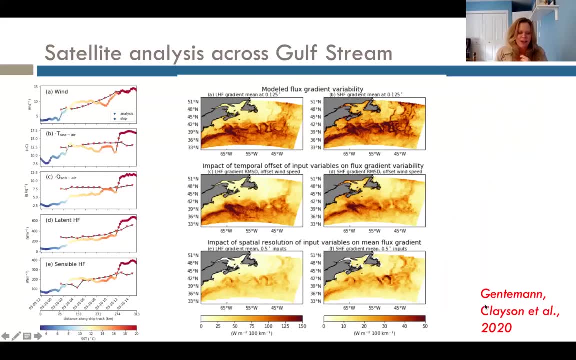 you're starting to warm the lower part of the boundary layer And then, as you get to the warm side of it, just how much deepening that's a 1000 meter mixing on the warm side of that front. Okay, And one thing that we have tried to look at is: what do the satellites show us? And one of the 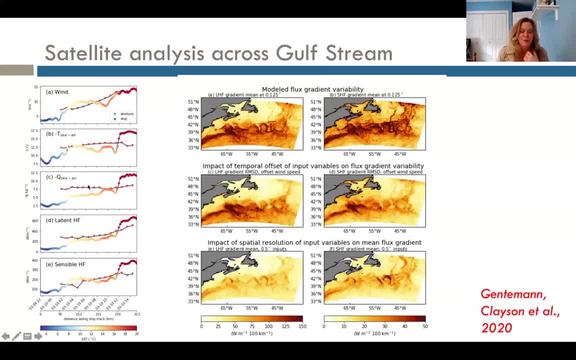 things that we're finding is that many of the SST products that we're using for doing the fluxes, you know the winds, So the- again, the colors here are SST, But the solid line here is the ship's data And then these triangles are the satellite data, So it's kind of tracking the winds. 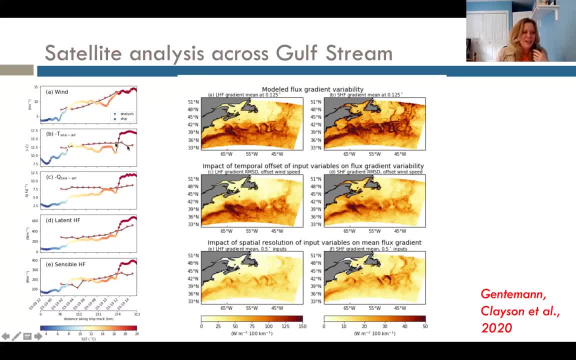 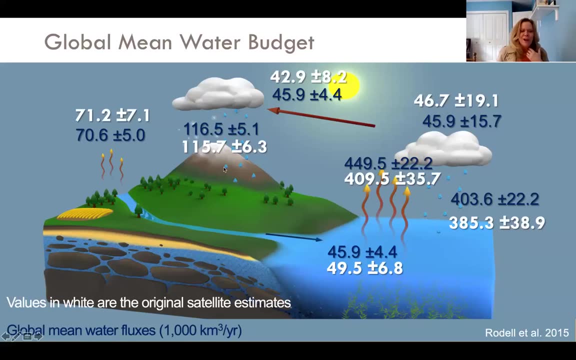 But the air-sea temperature difference is, you know, in the mean is okay, but we're capturing almost nothing of that gradient Which is a key, a key factor. So let me see, Okay, so I will just say that I should point out the global mean water budget. 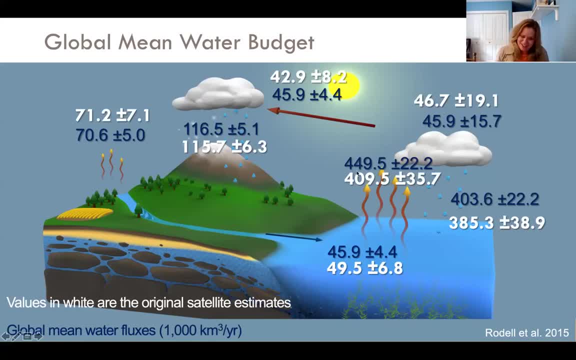 If we use the original figures. the original figures are, the original estimates are in white and the blue numbers are What we needed to balance the terms. you can see it was about a 10% difference between what we thought the ocean evaporation was, what our satellite estimate was and what it would need. 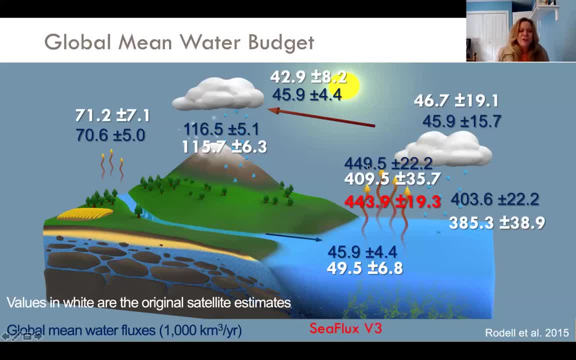 to be to be balanced. I will just point out, there's a new version of our flux product, which I'm going to show you in just a moment, And it's closer to the balance value, which is somewhere around 450.. And we're- we're definitely above where we were before, So progress has been. 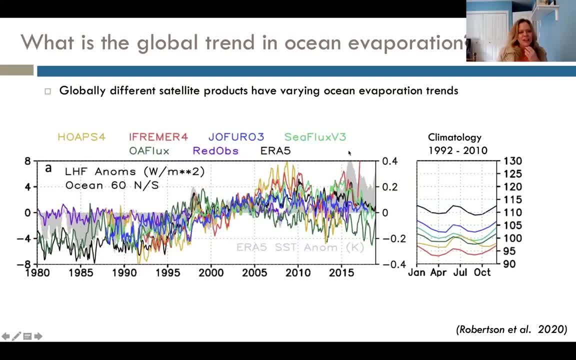 made. Okay, Okay, Okay. We really want to understand the global trend- and ocean evaporation. This is a number of different satellite products, So these colors are for different satellite products. always flexes, a blended product. Red arms are a series of. 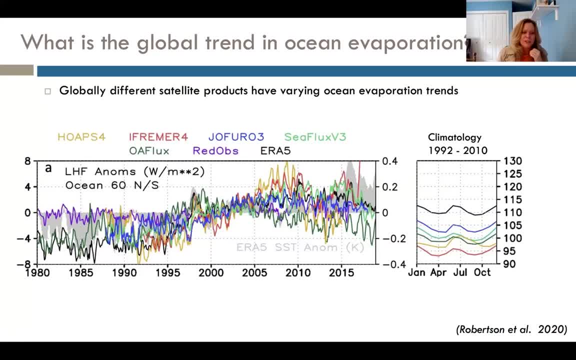 Models that use a very limited set of input observations to drive them. So this is now the anomalous latent heat flux from 1980 through about 2020, and I I'll just let you look at that and see if anything strikes you. 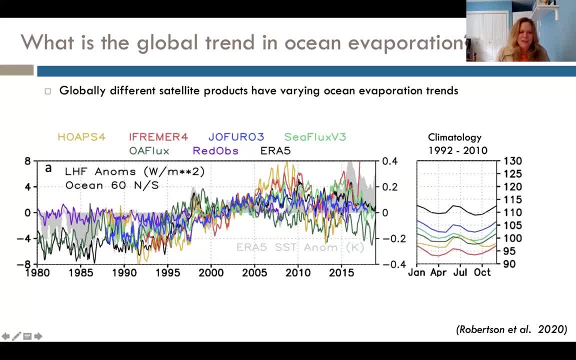 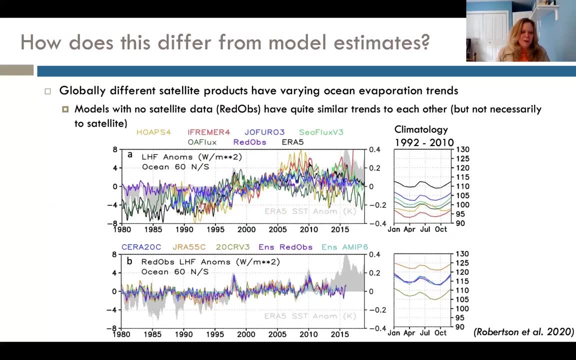 is it like a really consistent trend for many of the products and just the differences between them are kind of astounding. So trying to use them to understand trends, We still have a ways To go. um, and this is just the same figure, but now, with the, the reduce. 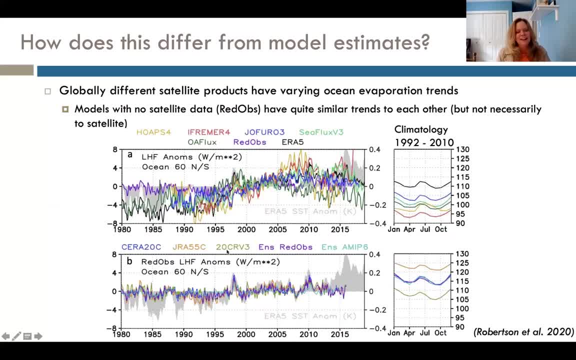 The fact that we're using the mean of these 3. Uh by Uh, Uh, the Uh models is- is not causing that lack of variability. They're very, very similar to each other- Um and uh- and all of them tend to be much higher in the 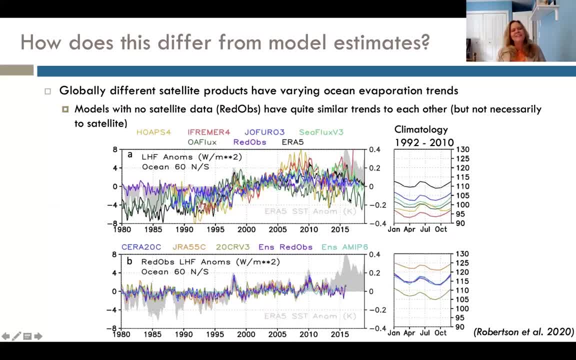 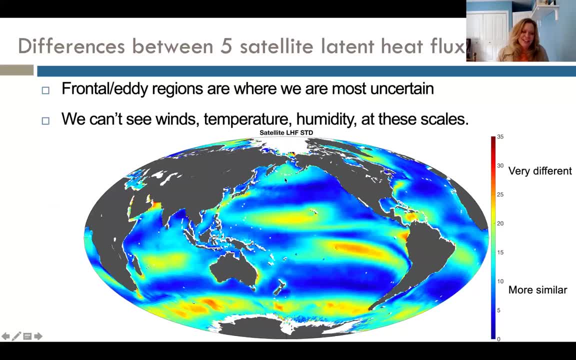 Even than the satellite products. so Well, some work to do. and if we look where the products are most different from each other, this is taking the 5 products and seeing where they're the most different. The red and the yellow is where they're the most different. 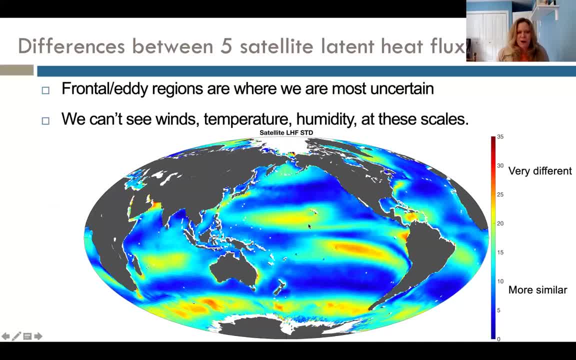 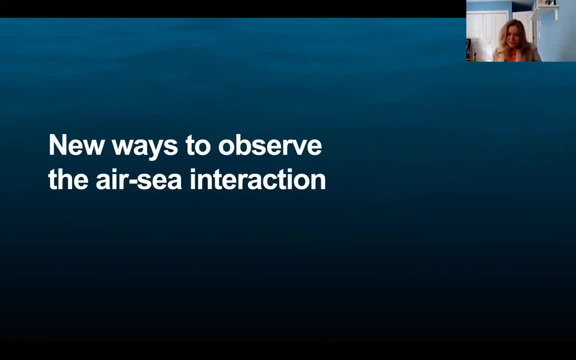 Often this is in the frontal or Eddie region where we are most uncertain, and that's because we can't see when temperatures scale. So I'm going to take about 5 more minutes and I'm just going to do a quick some of the things that we're doing to observe. 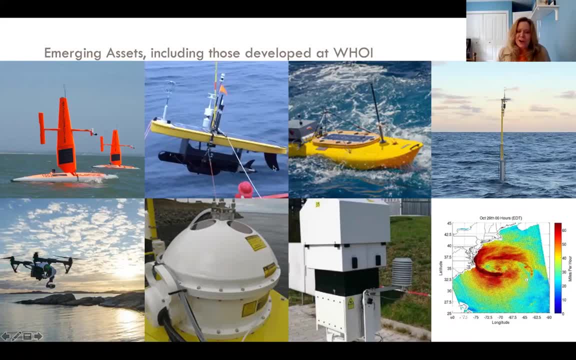 Air sea interaction, so a lot of it is autonomous. You know drones, things on the surface, Sail drones, wave gliders, working towards getting Um Better lighters of various kinds. This is something that I helped develop here. It's called the X bar. 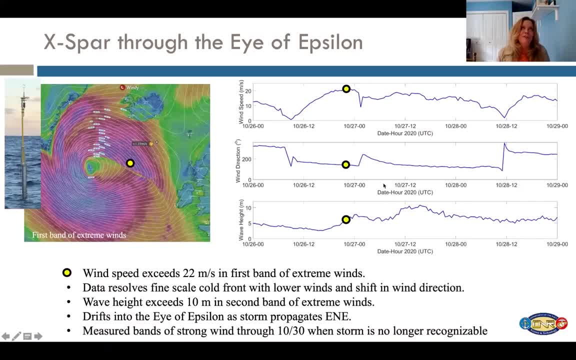 We'll look at that in just a moment. We put it out for the 1st, For a 1st long deployment this last winter in the North Atlantic, because why not take the most extreme Part of the ocean so it measures? you can see it sitting up in the water, so we can measure. 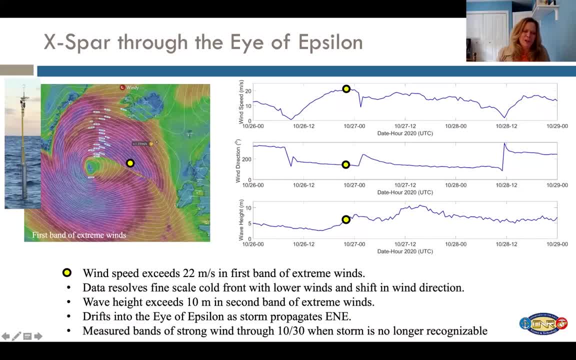 Um, it's actually directly measuring the fluxes, so it's getting turbulent. measurements of moisture, Um and when, and. and we just happened to be sitting there when epsilon Came came through, and so here's the wind speed, So getting 22 meters per 2nd in the 1st and when. 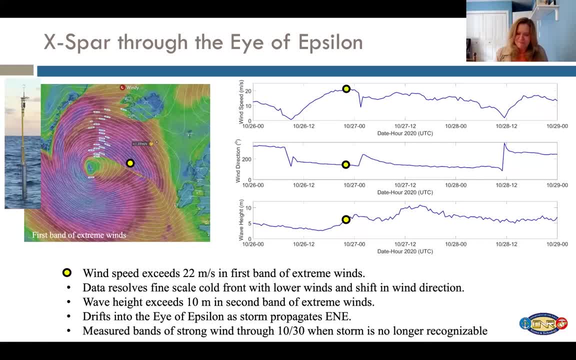 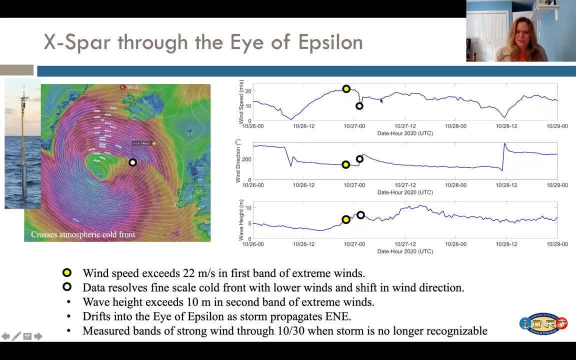 We're getting significant wave heights of 10 meters and as time goes by, that we can really resolve that cold That comes through their lower winds, a shift in the wind direction. There we go, the wave heights again exceeding 10 years And the next. 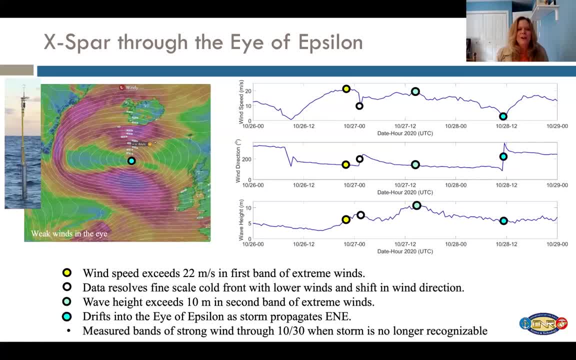 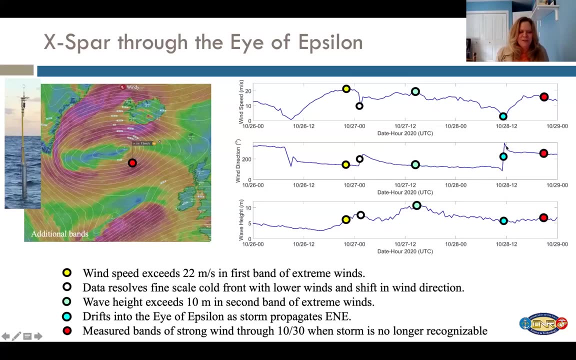 Band of storms and then we drift into the eye Of epsilon, and so the winds just pretty much completely died down. You see this in the shift in the wind direction And we we measured long, you know, various bands of strong winds. 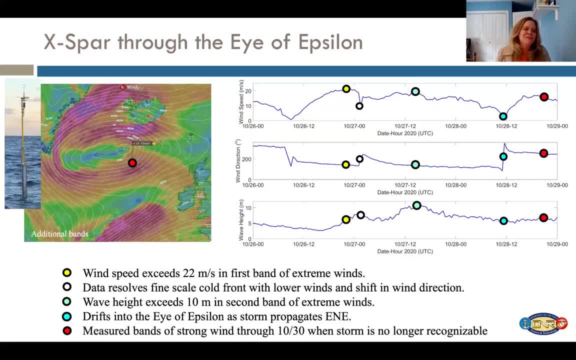 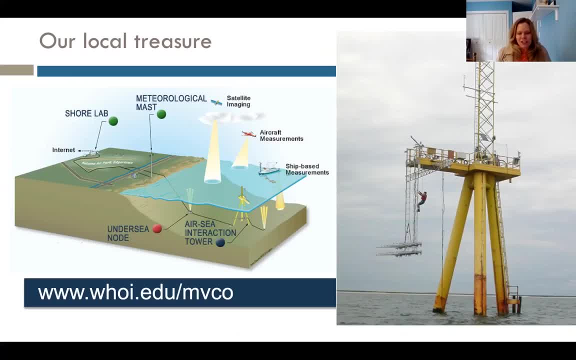 When the storm was no longer recognizable. so this is just an autonomous float that we put out. We have a local Air sea interaction tower- that picture of it on the right, just off of Martha's vineyard- That we have been utilizing to make a lot of high quality turbulence measurements, including the experiment where we're measuring fluxes within the atmospheric boundary layer and between the atmospheric boundary layer and the oceanic boundary layer. 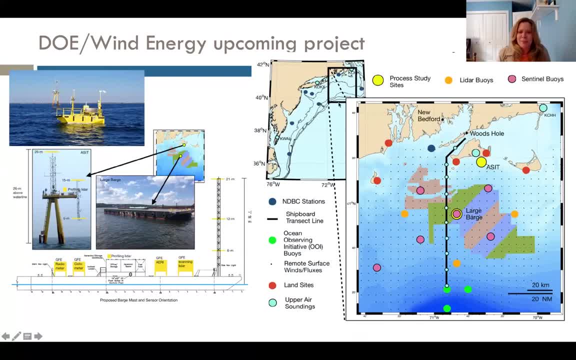 We have an upcoming project with the Department of energy, So this is now the same tower. It sits here. This is a map. There's Massachusetts up here And and Rhode Island. here's Martha's vineyard. So this is where the tower is. 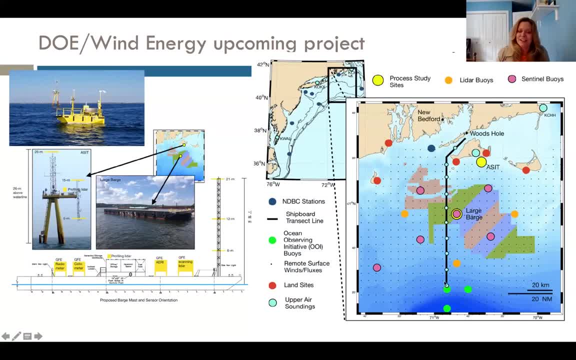 Pioneer I buoy array is down here. These colors are regions where the wind farms have Have leased out, and so we're going to do an intensive observation phase. We have light, our buoys that are being put out. We're having a barge with another tower on it being put. 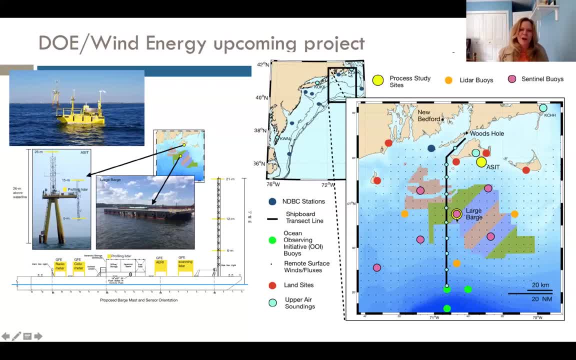 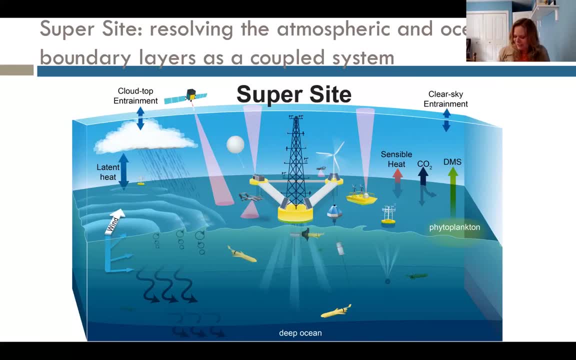 Out and trying to do a better job at really doing the coupled boundary layer system. The goal, of course, is to try to get some kind of System where we're really resolving the atmospheric and oceanic under layers as a couple of systems. 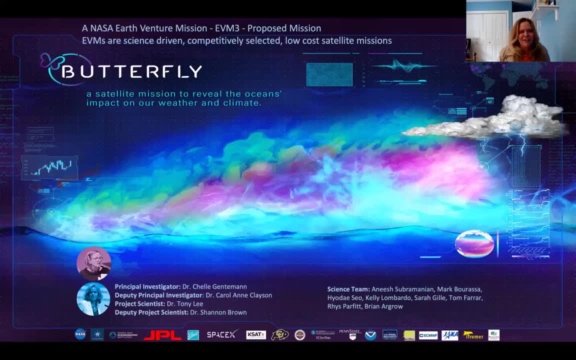 And the last thing, which was already mentioned, is our earth venture mission. proposal of butterfly, gentlemen, is the PI. I'm the deputy project scientist, with Tony Lee and our deputy project scientist, Shannon Brown. here We've got the close JPL with a number of other institutions as well. 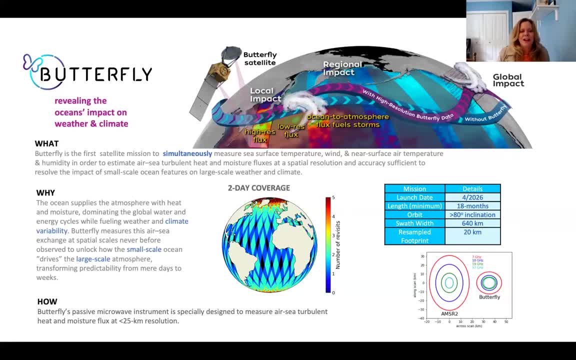 And the whole goal of this is to do a higher resolution And fully measure all the things that we need to calculate that latent and sensible heat flux from: 1. Satellite system at at less than 25 kilometer resolution, so that we can Look at not only how the high 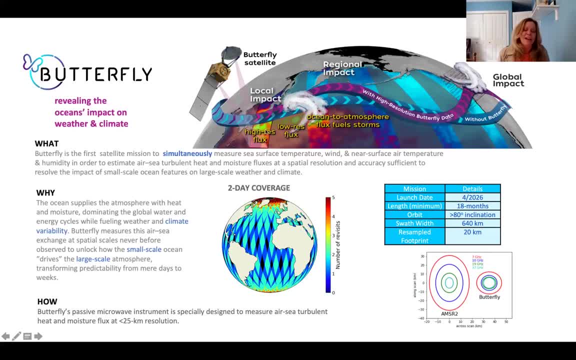 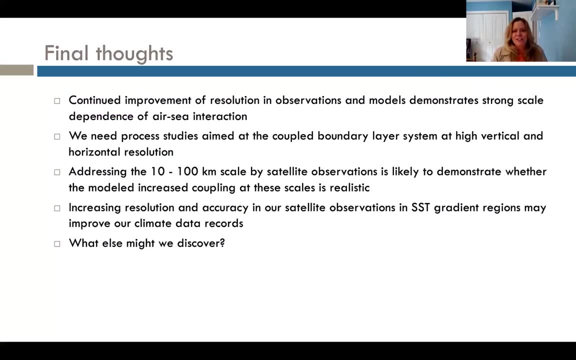 Resolution fronts and Eddie's impact back on our weather and climate, But also how resolving this may improve our, Our observations in general. so just some final thoughts. There's continued improvement of resolution and observations and models that demonstrate the strong scale dependence of interaction. We really do need process studies aimed at the coupled boundary layer system at high vertical and horizontal resolution. 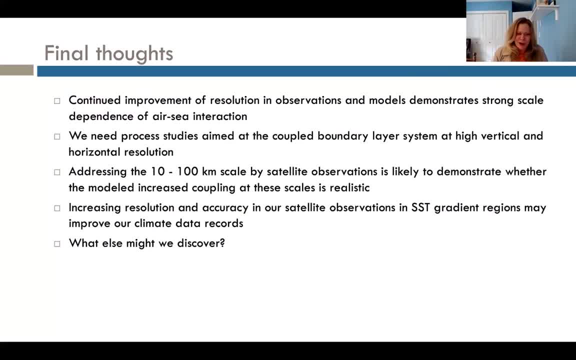 The models. the models are kind of outstripping our Our observations in terms of resolution and being able to address these with satellite observations really be helpful And might improve also our climate data records. and what else might we discover as we, as we keep looking closer and closer at this couple system? 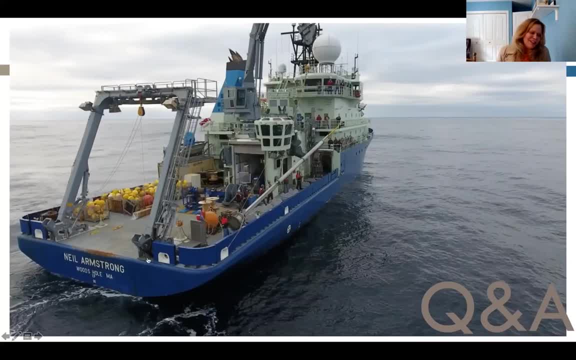 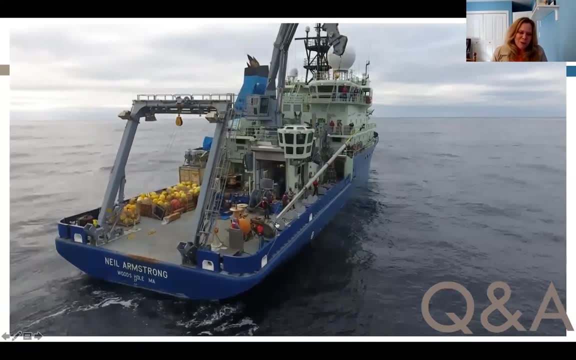 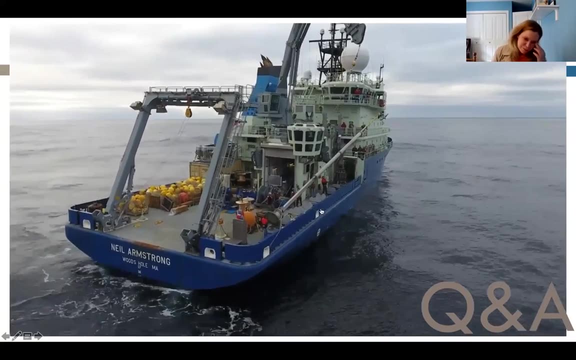 So I'm going to stop there. This is. I'm ready for any questions and questions that you may have for me. This is: This is the deployment of that X bar that I mentioned. I just want to give a shout out to the, to the team that went out on this. Not only did we have to do finish the preparation of the buoy under sort of conditions, to even go out on the ship. 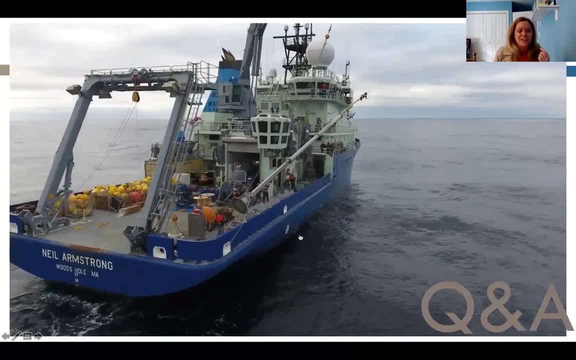 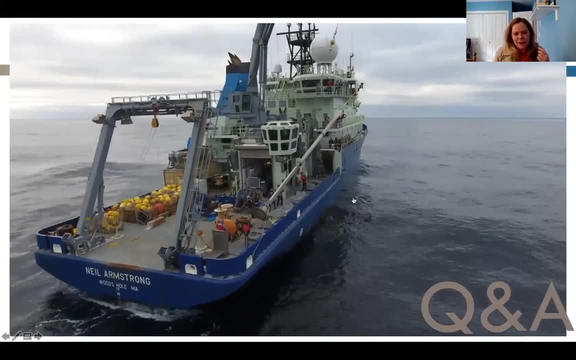 They had to corn a hard quarantine for 2 weeks before and 2 weeks after, So it was originally supposed to be a 5 week. Crews turned out to be 9 weeks total that they were, that they were gone. So I'm just going to leave. let that play, as you can see. 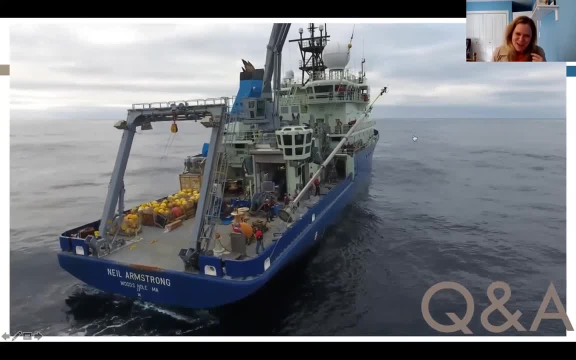 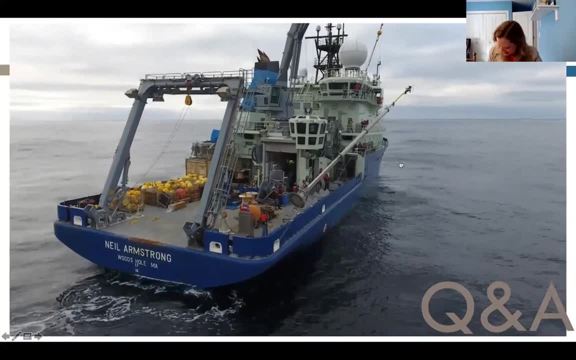 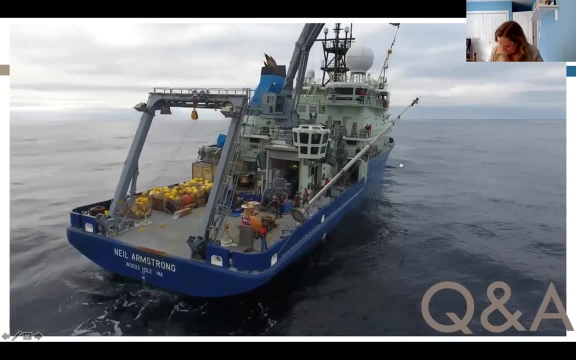 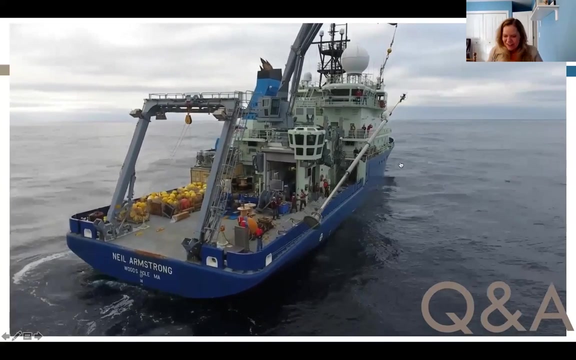 putting out these 14 meter. you only saw the top half of it above, above the water line in the pictures. I'll let that go and see if there any questions. Thanks very much. I actually can't even watch that video because it makes me feel a little bit. I have a video where that a colleague took when they were down in the southern ocean and I was. I was explaining why certain things were happening and it's from the bridge. 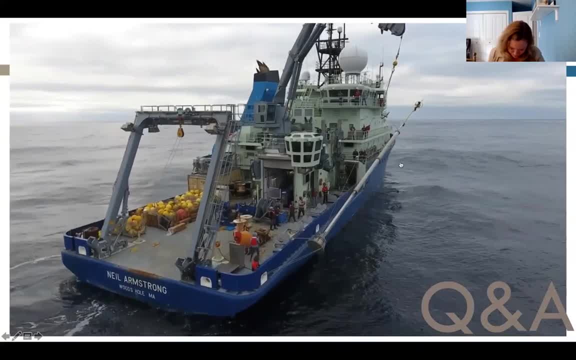 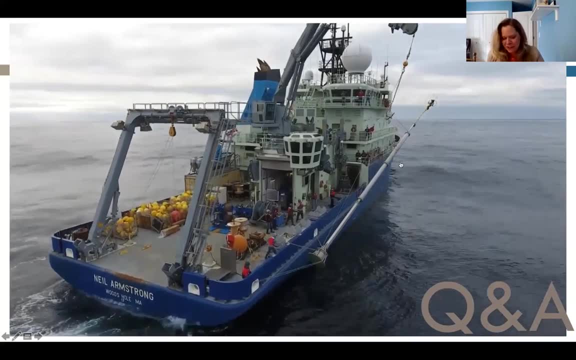 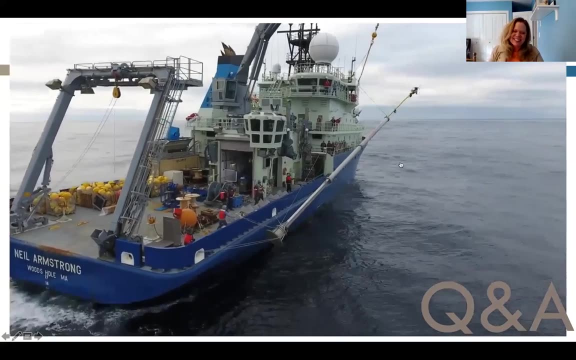 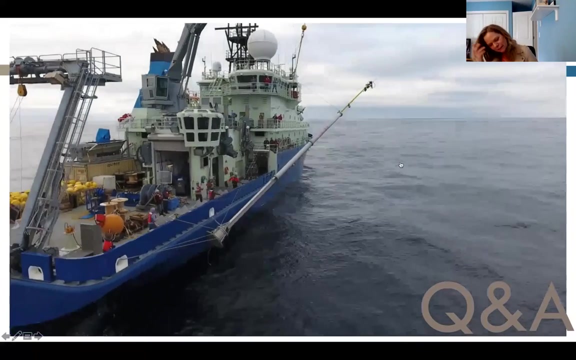 And I was doing it And it's show something for Teachers, and so it was, and teachers got up afterwards and called it the vomitorium of a video. So I'm going to hide that. We do have a question in the in the chat. Thank you very much for that, By the way. you know there's. you know it's hard. We all would love to be applauding that. That was very interesting and very. 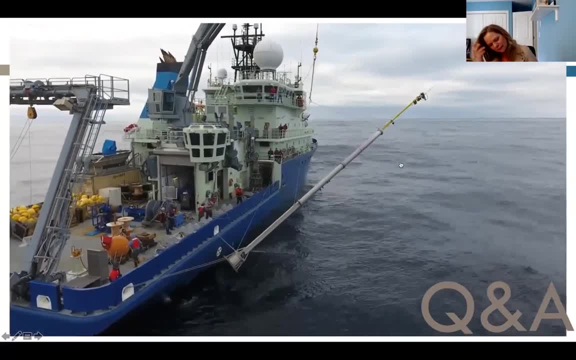 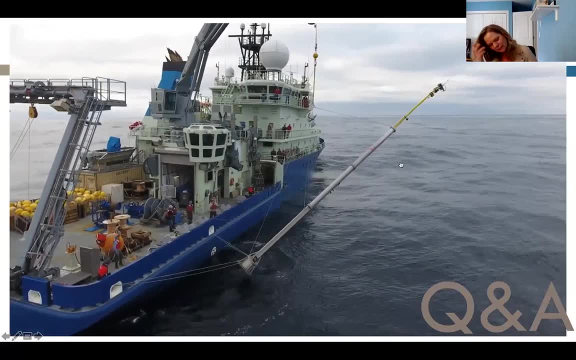 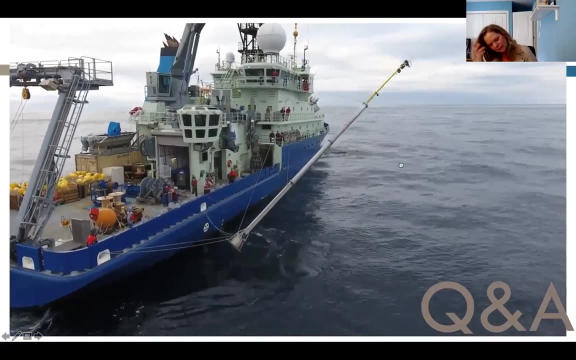 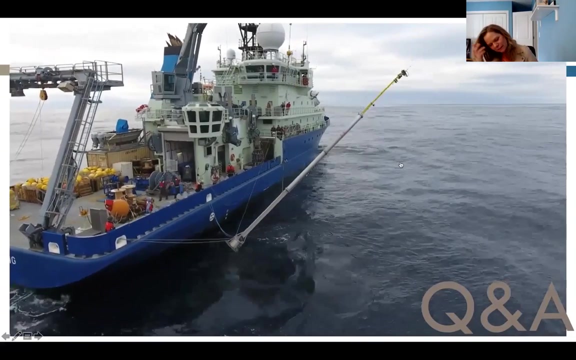 Accessible and very, Very thorough, But we do have a question from Evan Fishbein and I will actually two questions, but I'll read, read the first. I'll read them both And you can answer as you wish. The ocean heating is the difference between shore wave, long wave, sensible and latent heating, IE heat deposited into the deep ocean. First question: 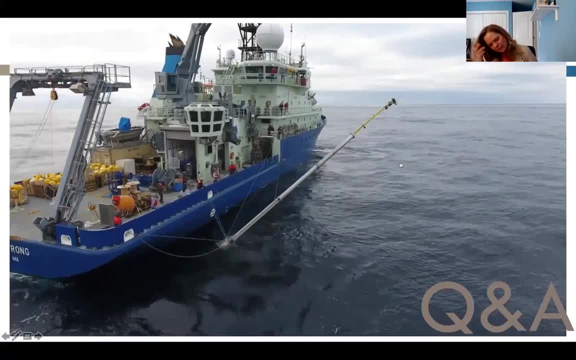 And then the next question is: does the MJO simulation include precipitation with changes in near surface salinity? And then the next question is: does the MJO simulation include precipitation with changes in near surface salinity? And then the next question is: does the MJO simulation include precipitation with changes in near surface salinity and wind gusts from precipitation? 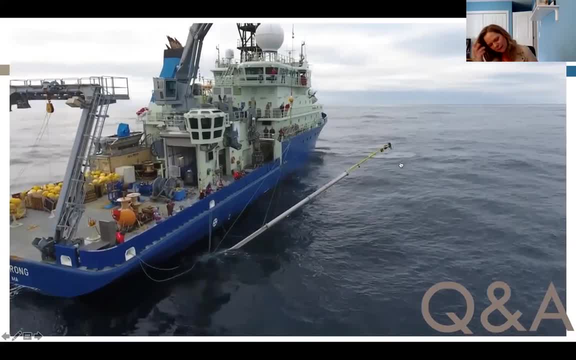 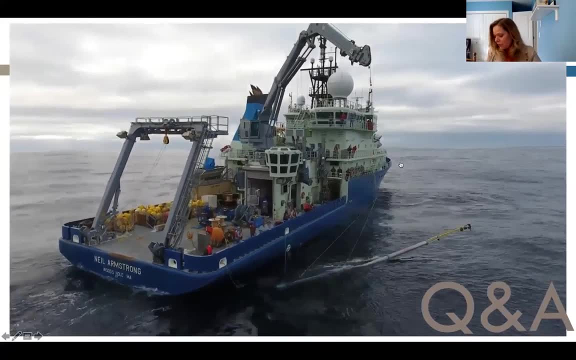 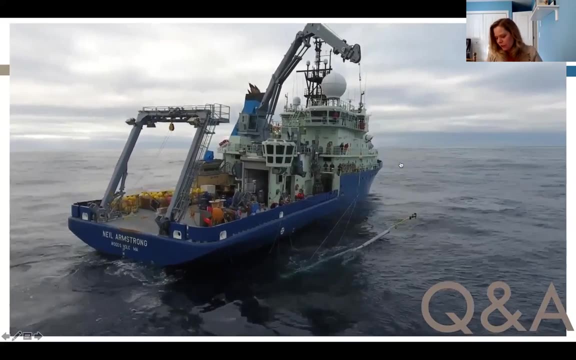 Yes, Okay. So to answer the 1st question, Yes, So the the, the ocean is gaining the heat through all 4 of those flexes that you 7 that you've mentioned, but shortly, All 4 of those impact onto the, onto the ocean. 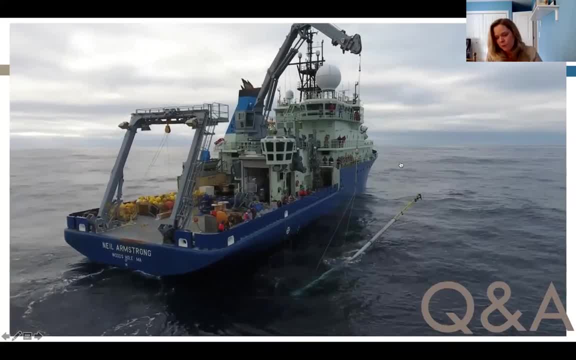 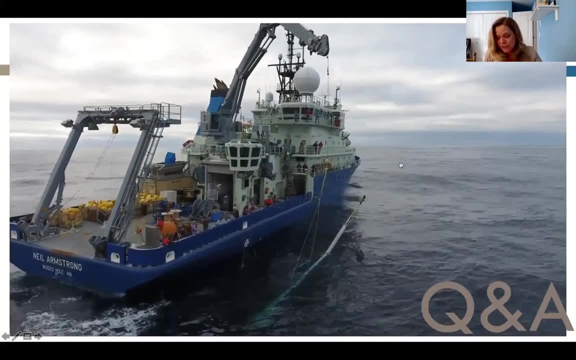 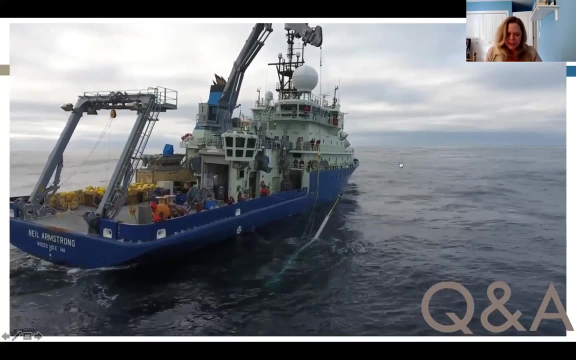 And the 2nd question about the MJO. it was a fully coupled model So that changes in salinity in the upper ocean- Um, Um- did impact back on the sea surface temperature, You know, through a reduction in mixing that, then that change in SFC was then included. then to changes in convection and precipitation. 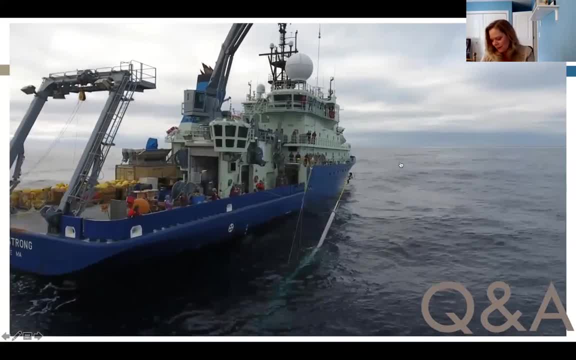 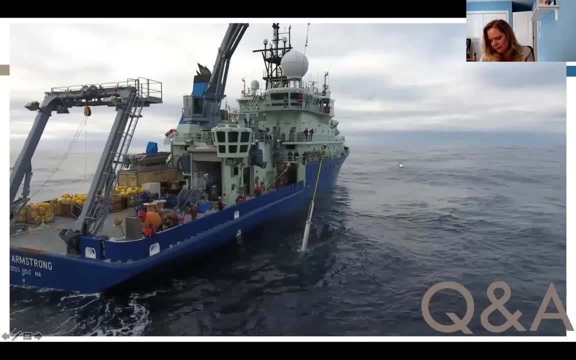 There's a question from Ben As well. I don't know if you want to unmute now. I know that I can't do it, typically He's got audio issues. I'll go ahead and ask it from Ben Holt: Have you encountered biogenic flicks in your field Work And stuff like that? 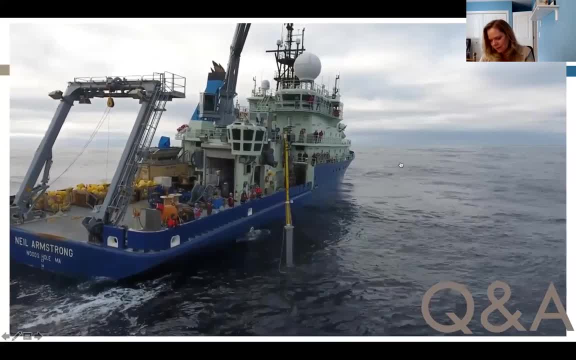 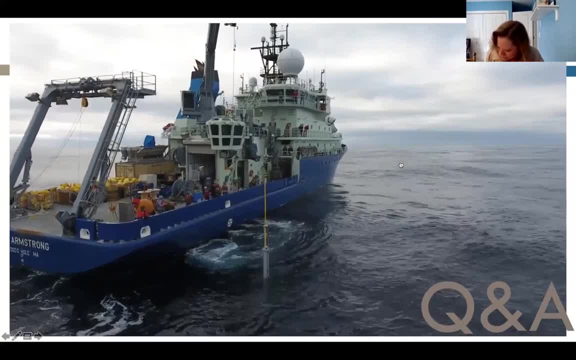 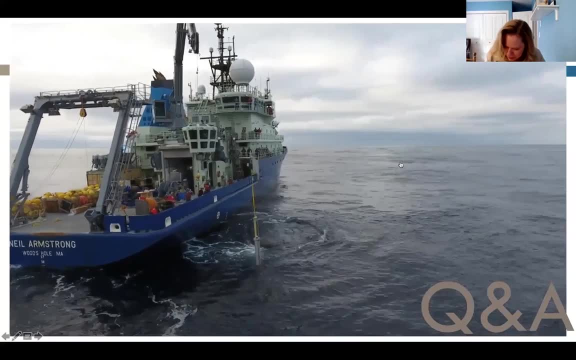 I'm sorry, can you ask that again? So biogenic: Have you encountered biogenic flicks in your field work, studies and notice any impact on air, sea fluxes? So that's a really good question. So in fact then, 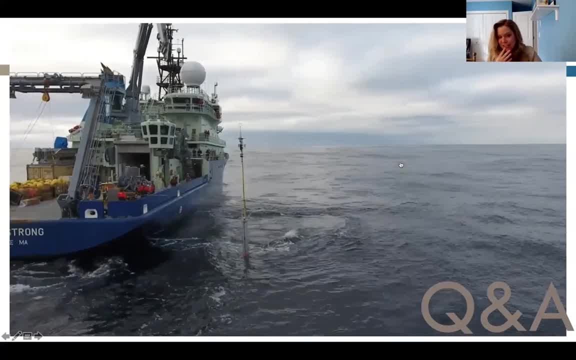 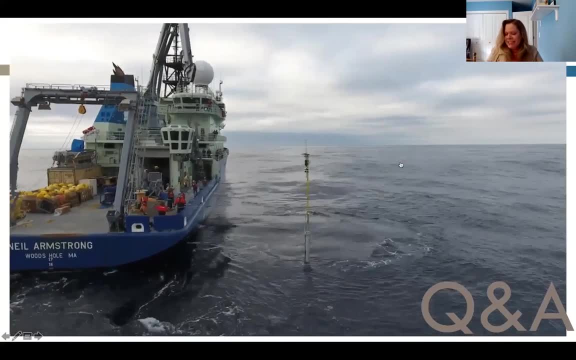 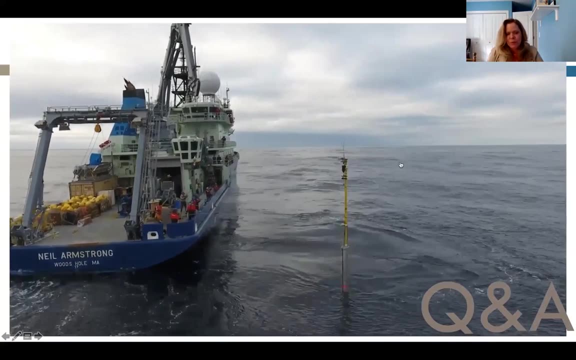 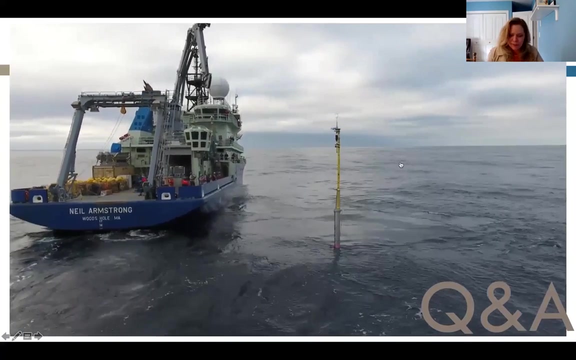 How, how those impacts that they, they do, And there is some work on that. It it probably does. it doesn't seem to impact it And you have to make a global scale variation. But they, they can impact back on the fluxes in several ways. And 1 is any changes to stability of the upper ocean. 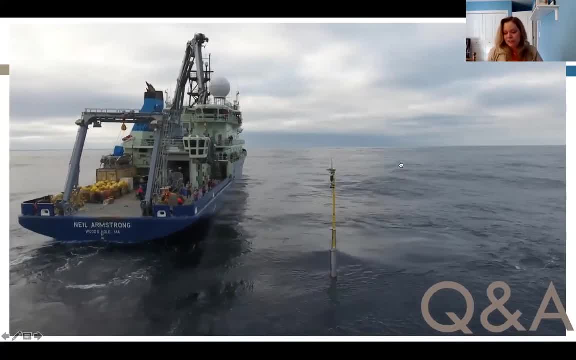 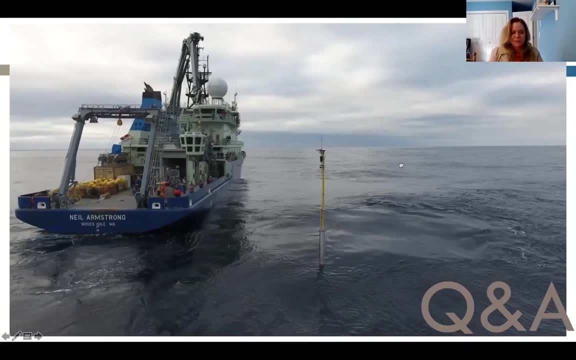 We'll change. you know, see surface temperature and also anything that changes the roughness Of the ocean. surface changes both how the heat and moisture exchange, but also the momentum exchange as well. So it is it definitely takes. It definitely takes a lot, a lot of different observations to fully look at how these are interacting with each other. And that's that's probably 1 of the most difficult aspects of it is to really capture all of that. 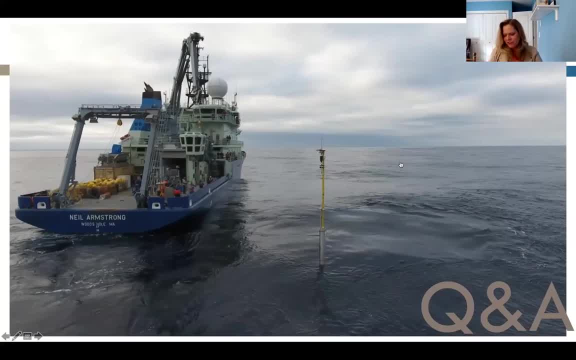 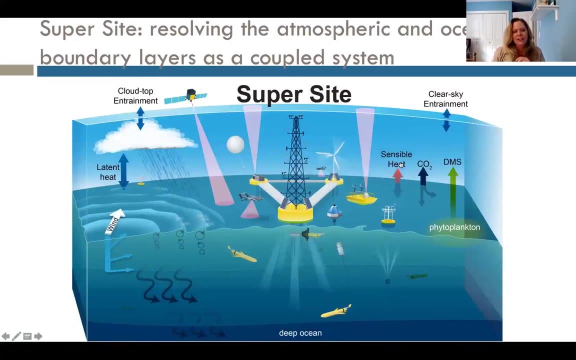 If you need a sort of a complete physical, biological, chemical, high resolution vertically and horizontally, And so, and I so I skipped over. Okay, Oh, we've got the X bar. you know that is. This is actually I proposed as an ocean shot to the national academies to be long term, what we're calling super site. 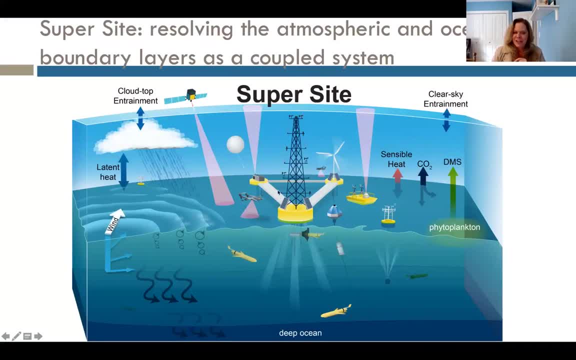 Better. you know they're taking advantage of, like moving wind turbines and where we are with autonomy now and trying to capture as much as we can, sort of coupled system as a whole. So, but that's one thing, So I'm going to stop here. 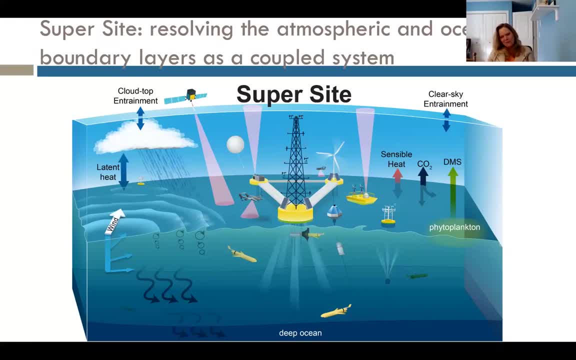 I'm going to put it in the chat, Okay. Okay, I'm going to say myself that I think you're going to need to give a solar array on your butterfly satellite. There's a question from Jorge Carol. thank you for a great presentation. 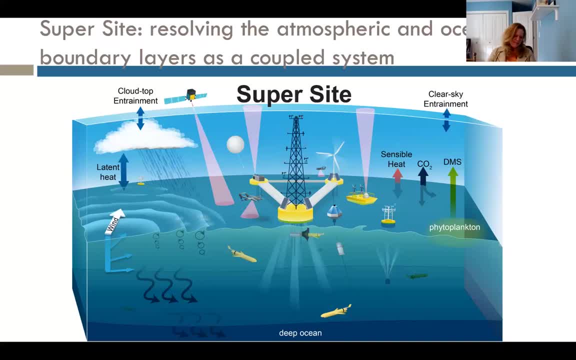 You think it would make sense to identify time periods when one has clear infrared imagery And do the gradient calculations and flux comparisons? Okay, Okay, Okay. So next question is from Sarah, Sarah, So this is a question for you. 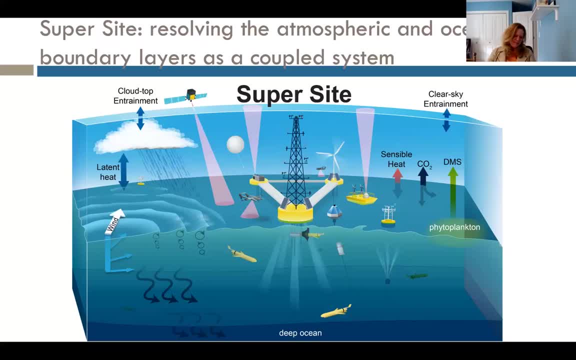 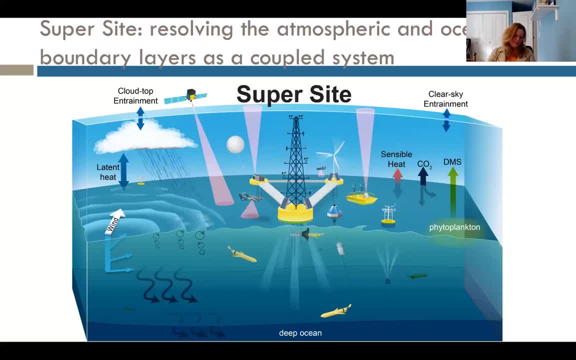 and do the gradient calculations in flux comparison. My concern is that there can be periods of times when cloud cover prevents calculating the full resolution of the SST gradient. Thanks, Jorge, Yeah, And you know quite well that 25 kilometers is not the best resolution we can do in SST. 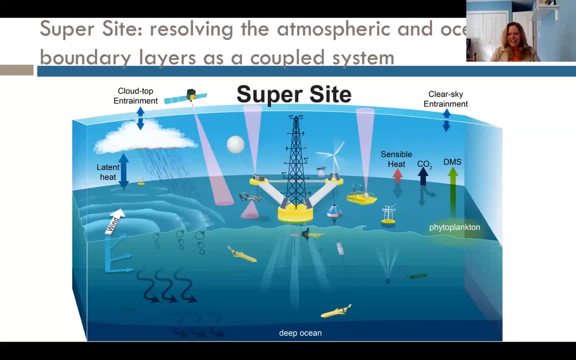 right. It can be much better than that, And one of the issues is that sort of the flux products themselves need a complete and entire sea surface temperature field, And so it tends to use either a- you know, vis-a-vis our- you know- microwave blended. 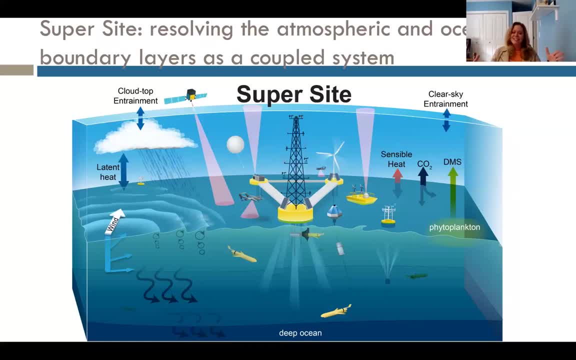 or just simply a microwave product. So, yes, we're looking at sea surface temperatures that are, you know, 25 kilometers, And if they're blended, then often it's. you know, if you're using the Reynolds, you're using the Reynolds, it's kind of optimally interpolated and so you're continuing to. 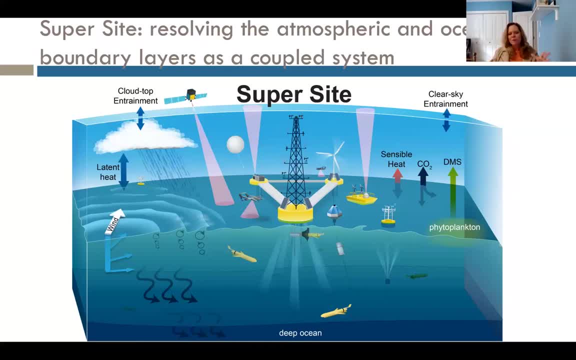 sort of smear out the ocean surface. So one of the problems is that we can do much higher resolution on the sea surface temperature but we can't do much higher resolution on the other components. So we're sort of at 25 kilometers for those values. 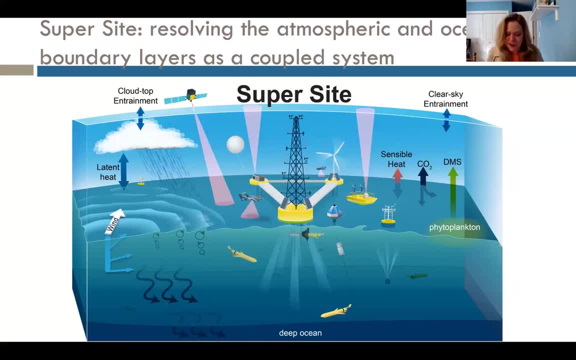 We are working on, and I know that some of you, even on this call, can do some tricks to try to get, like the winds, down to, you know, the sea surface temperature. We're actually right now trying to play around with a high-resolution version of SeaFlux. 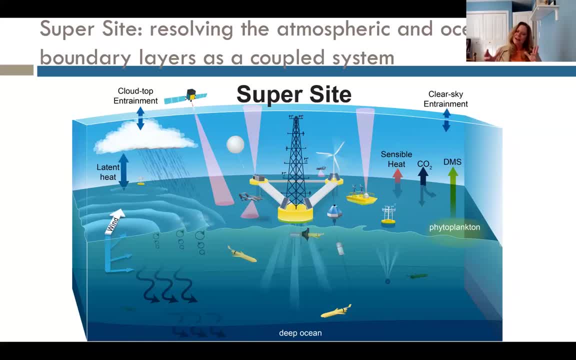 in which we use a higher-resolution sea surface temperature, and how, if we use that in combination with even the 25-kilometer air temperature and humidity field, does that show something a little different? Good question. Okay, Evan, do you want to go ahead and ask your question? 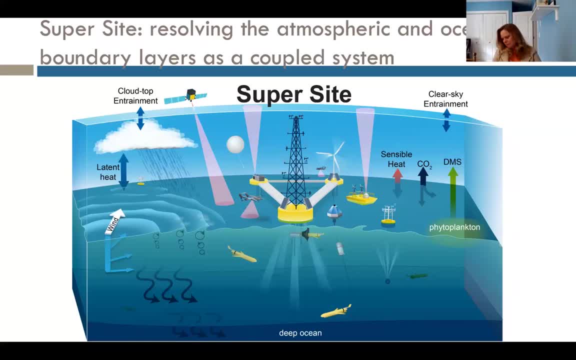 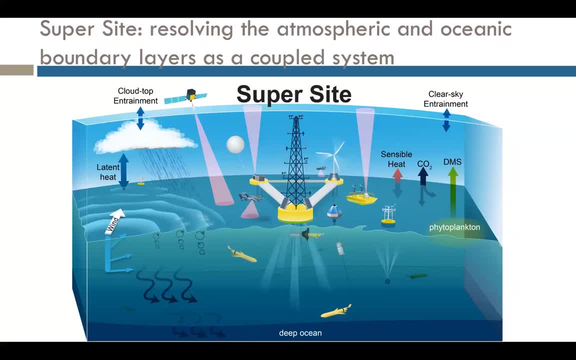 it may have been addressed by one of these maps you showed, but the question is: during the first decade of the 21st century there was sort of a hiatus in warming and my understanding is that's attributed to the death of the ocean. 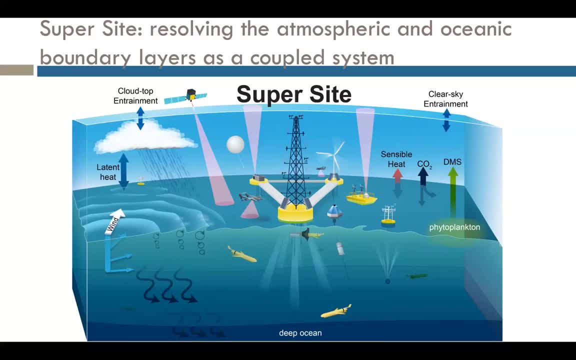 And I was wondering if you have a feeling for where, if heat gets transported into the deep ocean, does it tend to occur in eastern boundary currents or western boundary currents or in the tropics? So that's a good question, And I'm thinking that when I I haven't looked at that like any the most recent work, that's. 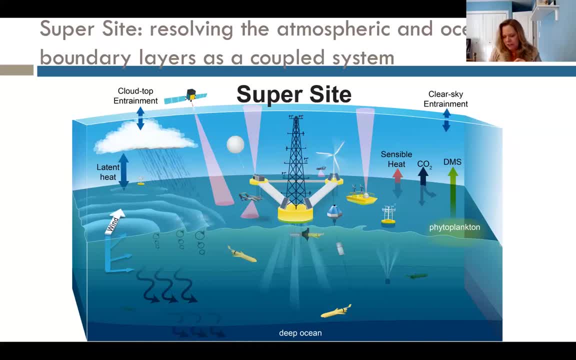 been done on that. So I'll just give it as a caveat A lot of that. that exchange seemed there was a lot of focus on the tropical Pacific for where that, where that uptake of heating might be, And you are absolutely right that one of the discussions or one of the possible causes 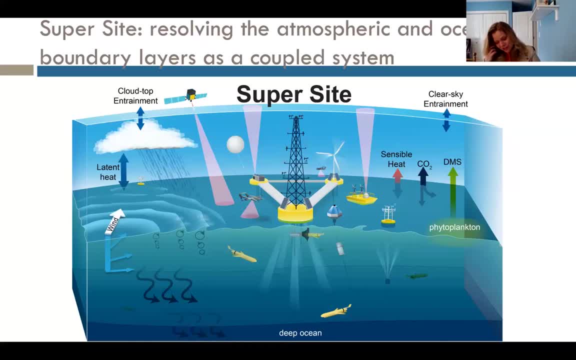 of the hiatus was you know that just that the deeper ocean was taking up more heat than the upper ocean And there does seem to be, you know, some change associated with that, And that that is one of the, that's one of the possibilities. 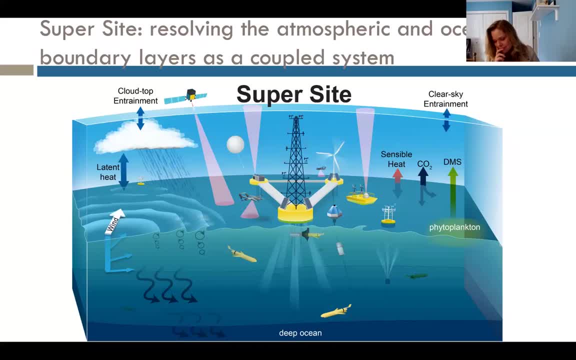 Okay, But don't you get greater in the eastern boundary currents? don't you tend to get greater, stronger upwelling? And wouldn't those be the places where- mostly where you'd probably be most able to transport heat into the deep ocean? 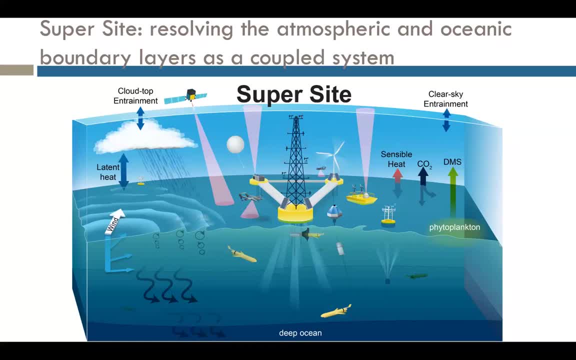 Well, the best places for transporting heat into the deep ocean are the, actually the deep convection. If you really want to get to the deep ocean, that's where you get. you know, convection down to a thousand meters or more of that. 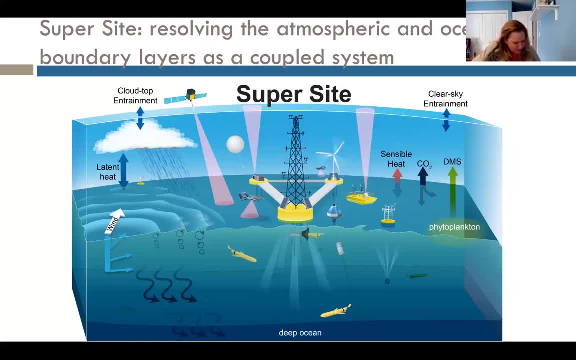 But it in terms of where you might have this heating. some of it has to do with it as you change or change the trade winds, So you have differences in Ekman pumping. excuse me that, that will. that will make an impact. 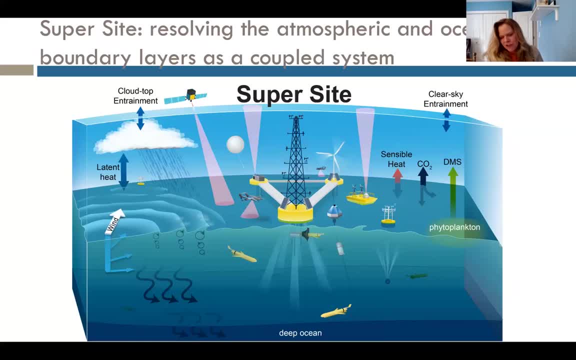 And I mean there's there's a number of dynamics that go into that And it we really are talking about things you know, more than just sort of the very upper ocean now and getting the getting the heat down deeper. 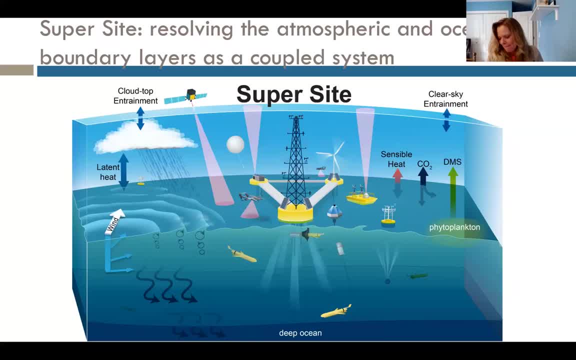 So I just want to thank you for this talk. The only problem is it's actually a semester long class, not just a one hour seminar, but it was very interesting. Thank you, Kevin. Does anybody have any other questions they would like to ask? 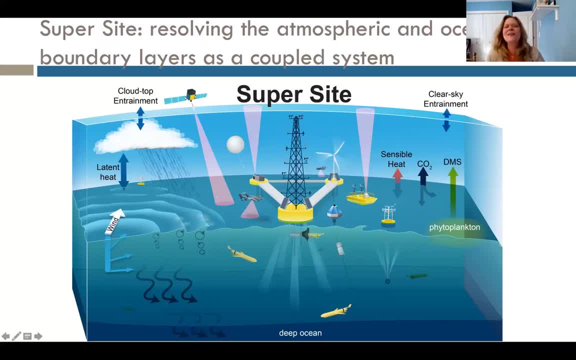 You can unmute yourself. I know that you have a number of other talks or other meetings today with some groups and individuals, but in case somebody has a question they want to ask now: Hi, this is. this is Ron. Can you hear me? 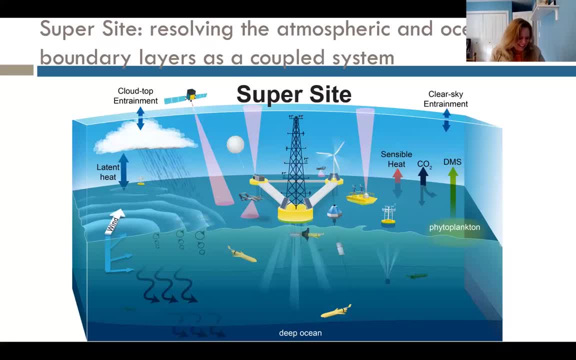 Yes, Yeah, Just thank you for the wonderful presentation. It was great. Looking forward to meeting later on and I hope you enjoyed the meeting today. Thank you, Did you have a question? I have a lot of questions, but I'll ask it when we meet. 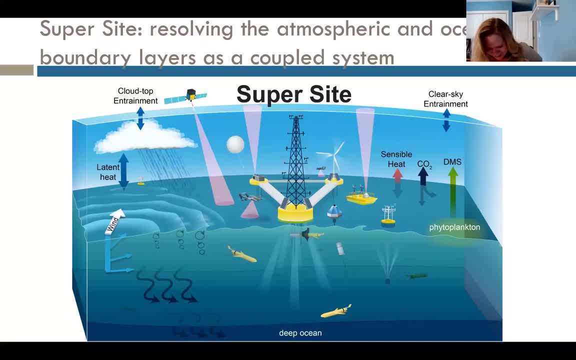 But I just wanted to explicitly thank you for the great presentation and agreeing to do a virtual visit, which is, as you said, not ideal, but I think it's going to be very positive anyway. So thank you again. So I'll just call you out right now. 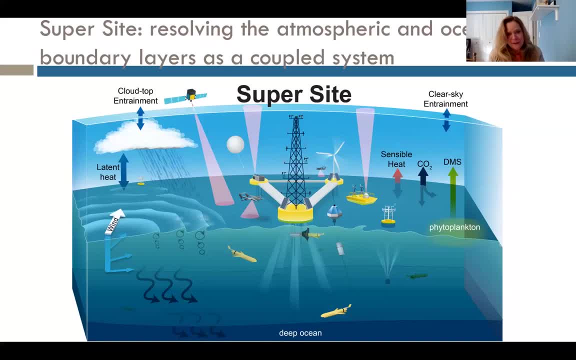 And thank you again for your leadership of the NASA PBL team And yay the release of our white paper. If any of you haven't seen it yet, ask you can send you the link for it. That was a lot of work and I'm hopeful that there's going to be a lot of great science. 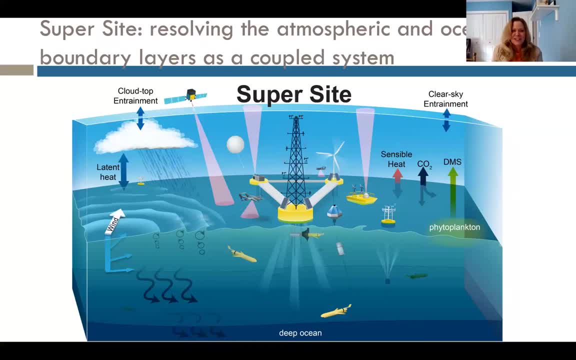 that comes as a result of giving this information to NASA. Thanks y'all. Yeah, thank you. Thank you, You're too kind. It was a lot of work for everyone. Thanks for your support. Hopefully people will find it useful. 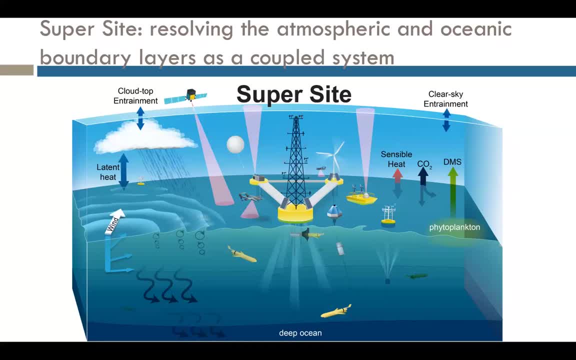 Yes, and having this virtual visit doesn't preclude a future in-person visit. So we have some, maybe some more results or something more to say about butterflies at some point in the future. You know we can Thank you, Thank you. 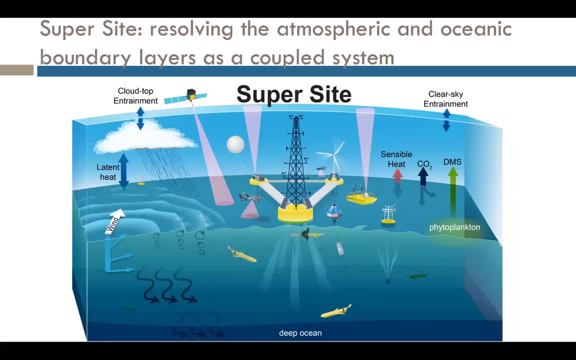